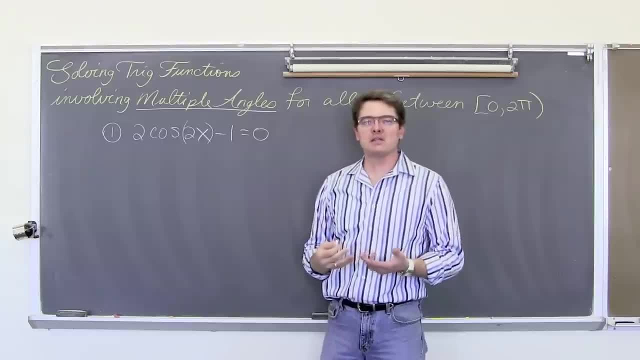 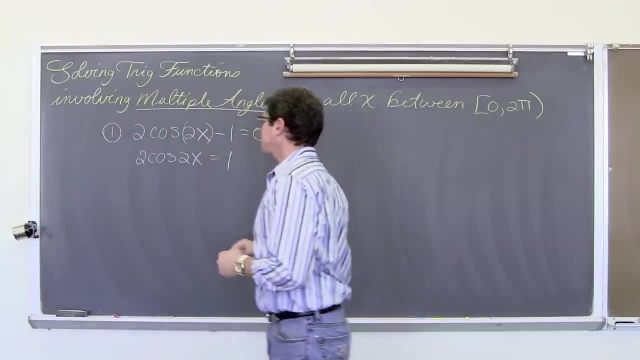 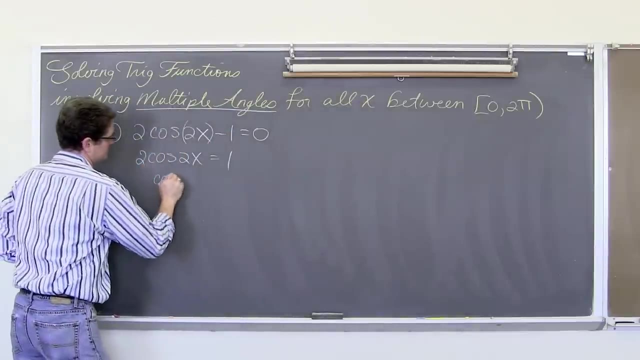 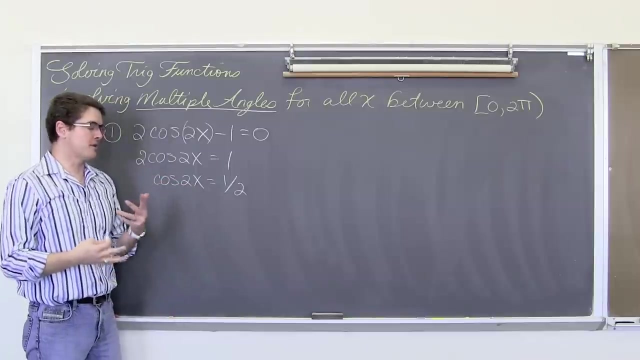 measure And you need to get two x by itself. Well, that means we are going to add both sides by one, Divide both sides by two, So I am going to do that multiplication of two. Now we have the cosine of two. x is equal to one half. Now, please remember that this is a trig. 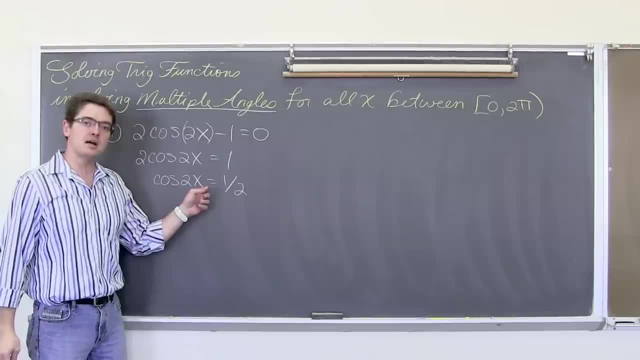 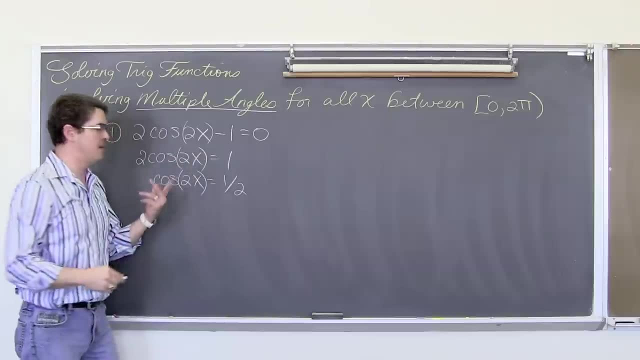 function. It is not just a variable. It is not cosine times two times x. We cannot just simply divide away this two. It is the cosine of two x. I like to keep my angle measures wrapped up in a set of parenthesis. not mathematically necessary, But it really highlights that it. 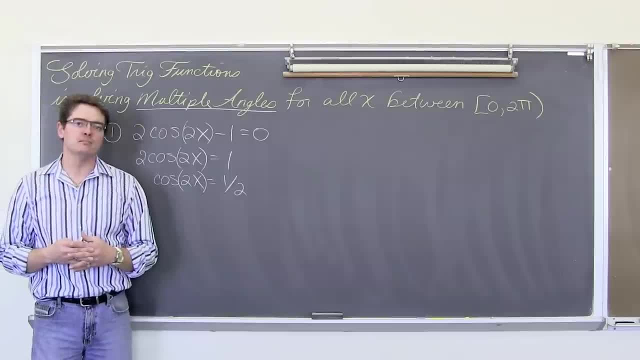 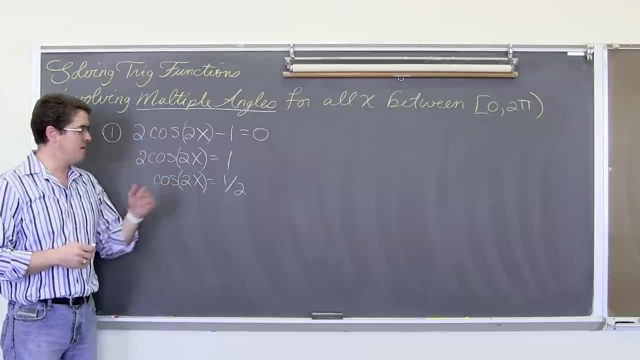 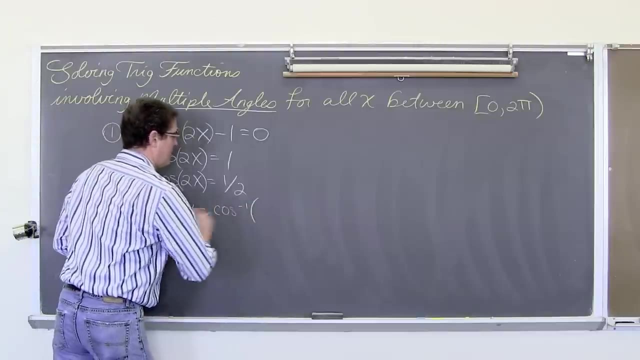 is a math function of cosine being applied to this angle measure. Now you want that cosine function to get away from the angle measure of two x, This double angle, And you want to do the cosine function by doing the inverse. So we have: two x equals the inverse cosine. 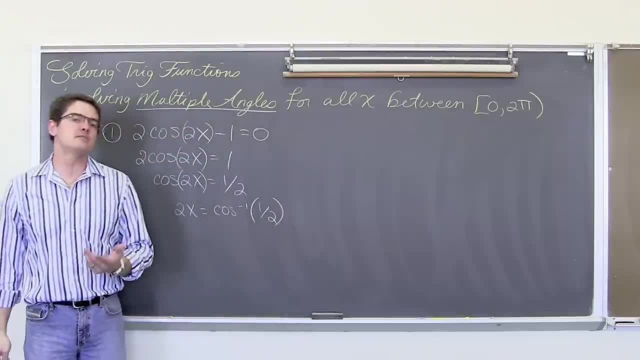 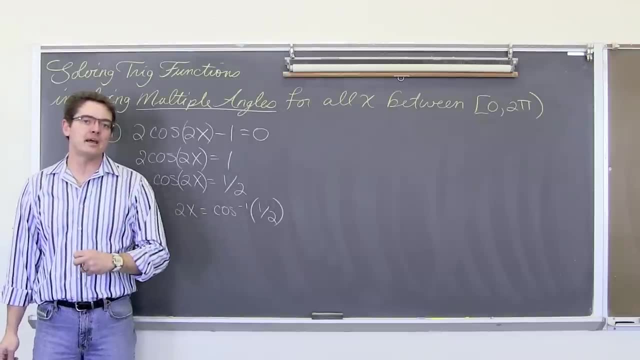 of one half. and don't forget, we put the sides of a triangle, in this case cosine being x over r, we put the sides of those triangles into the trig function and get out an angle measure. So again, if this is a brand new question and you have never done these before you, 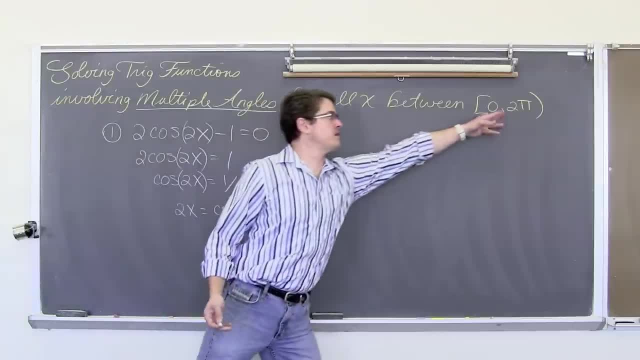 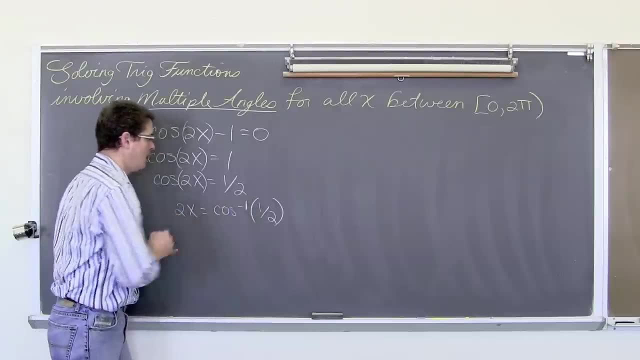 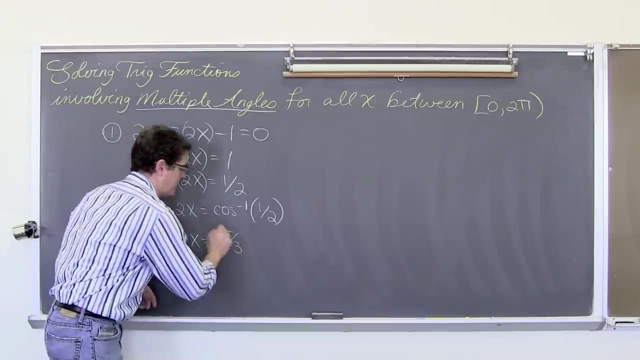 might be thinking: well, ok, again, the zero to two pi. where is cosine equal to one half? What is the answer to the inverse cosine of one half? Well, that is two. x is equal to ok, cosine is equal to one half at pi over three, and so pi over three, two, pi over three. 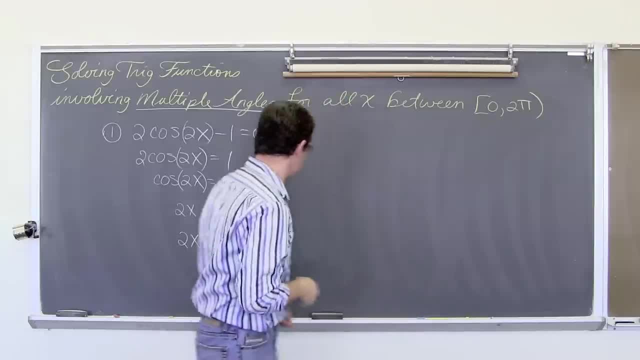 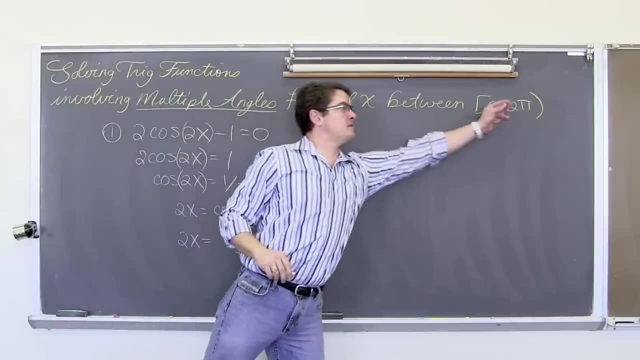 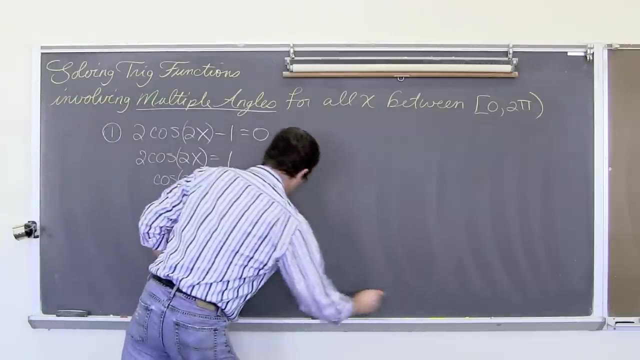 three pi over three. four pi over three. oh, that is right. five pi over three is the other one, And you might be thinking: ok, well, that is the two places on a one rotation of a unit circle where cosine is equal to one half, and you finish the question out by multiplying. 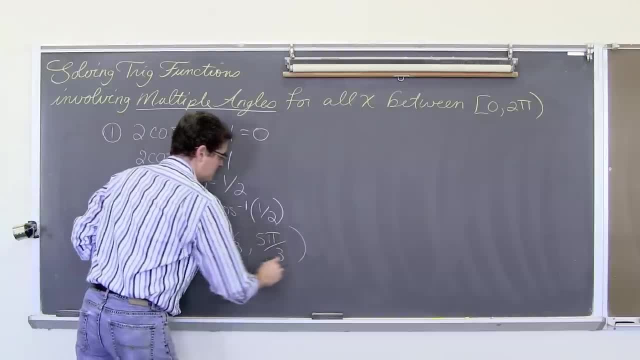 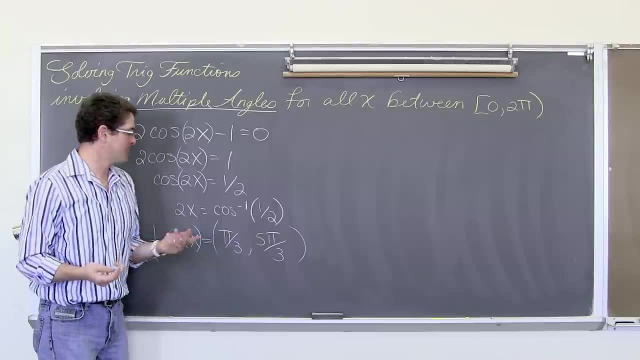 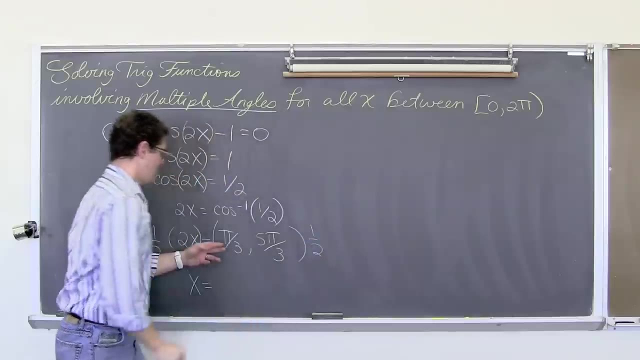 both sides of this equation by one half, Because We are not looking for trying to solve for the angle measure of two x, we are trying to solve for x, So we get: x is equal to one half of pi over three is pi over six, and 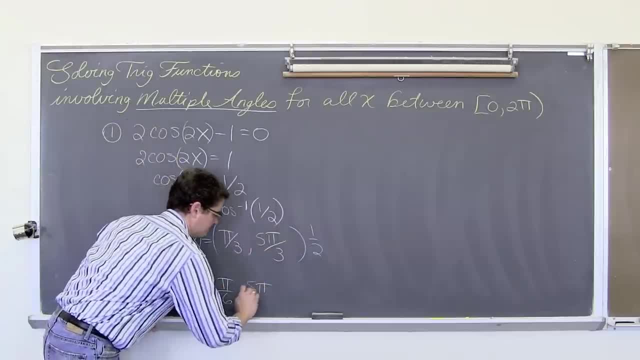 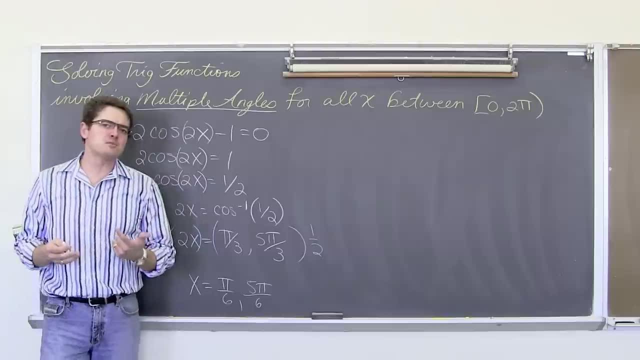 one half of five pi over three is five pi over six, So the direction set solved for x and I want all my answers between zero and two pi. But this is thirty degrees and this is one hundred and fifty degrees. I haven't even 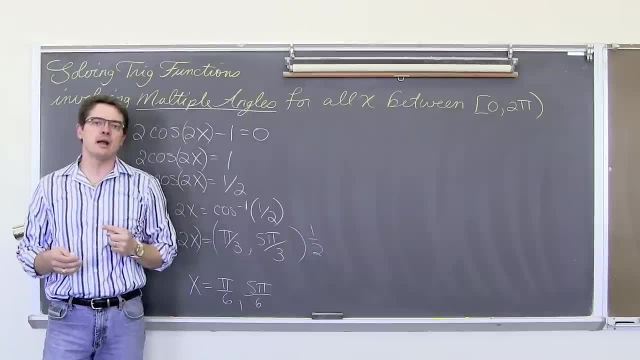 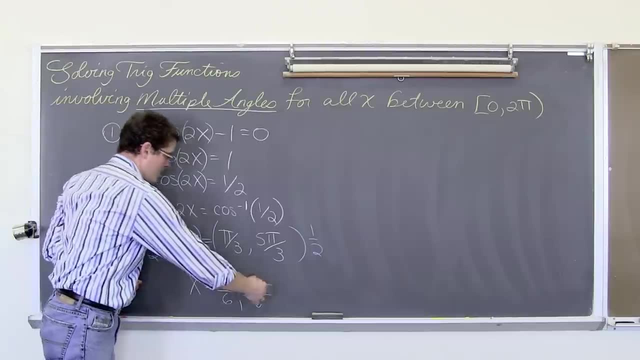 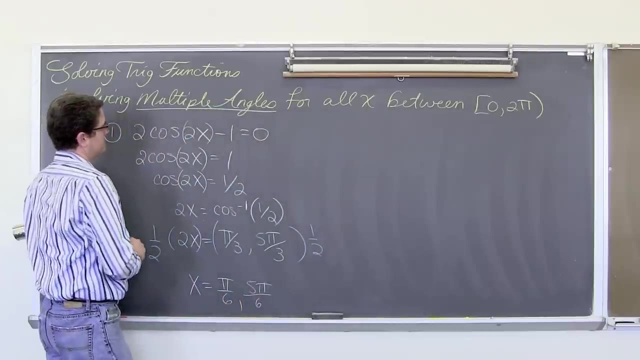 made it. I haven't even made it half way around the circle yet, So there might be some more possible answers, and indeed there is. See, the deal is, if you want all your possible answers, what you have to focus on here is this double angle And this two x or the 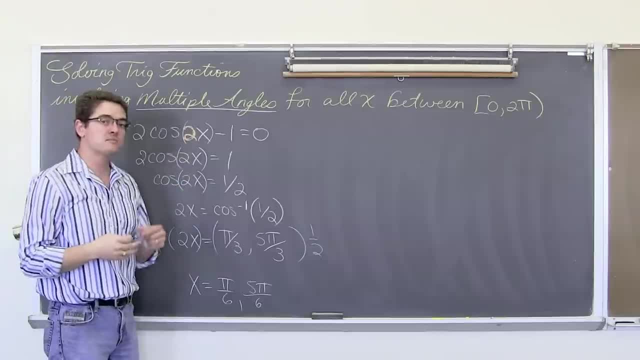 multiple that is in front of the variable you are looking for, the x. ok, that multiple that is in the x is equal to one half of pi over three, two pi over three, two pi over three. So you have to focus on the angle that you are trying to solve for That actually. 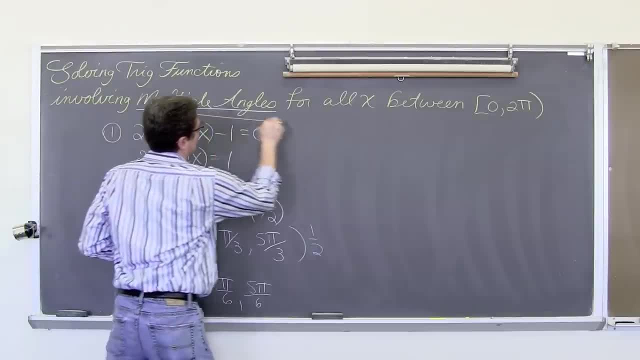 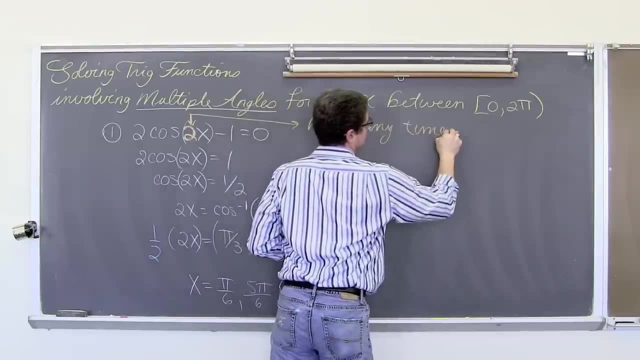 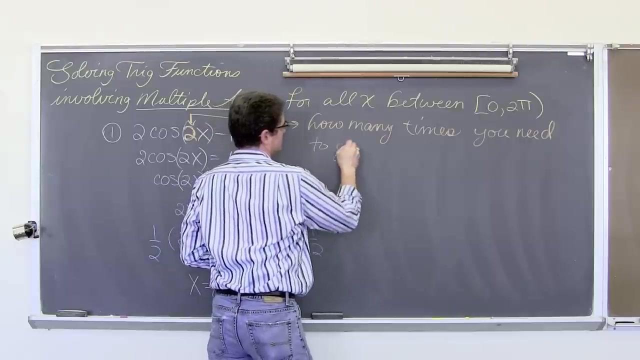 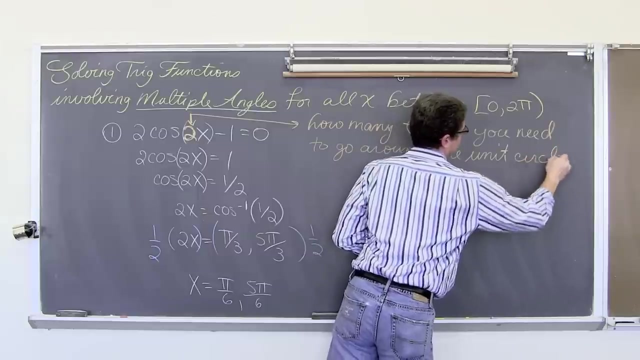 basically, you could think of this as how many times you need to go around the unit circle. You know, I just went around the unit circle and now I'm not sure how many times I have made it. You know, I just went around the unit circle and now I'm going to go around the 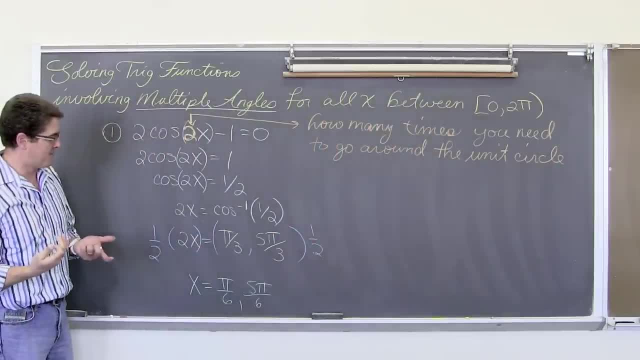 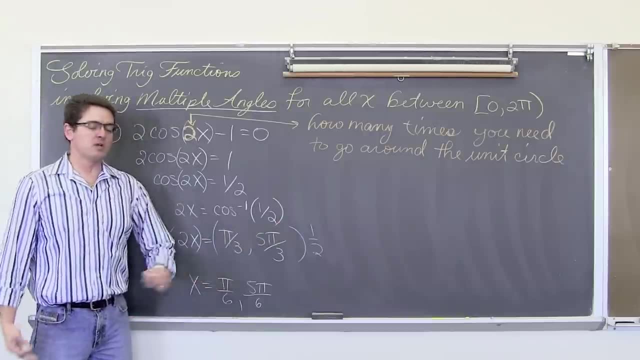 around the unit circle once, like we normally have ever done when we deal with trig functions. When I took that last step of dividing both sides by 2 to get x alone, we actually got some relatively small angle measures. They are correct, but they are not all of them. 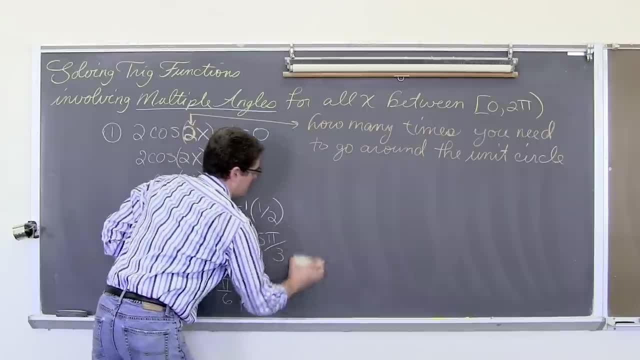 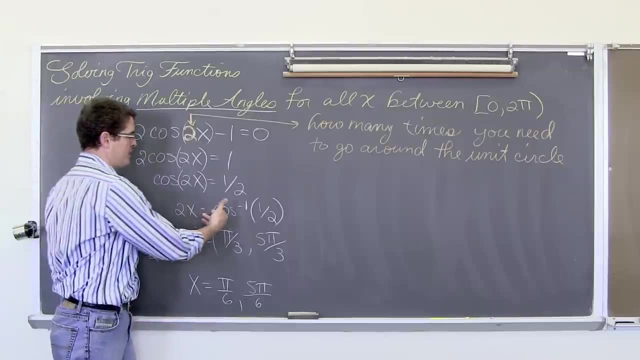 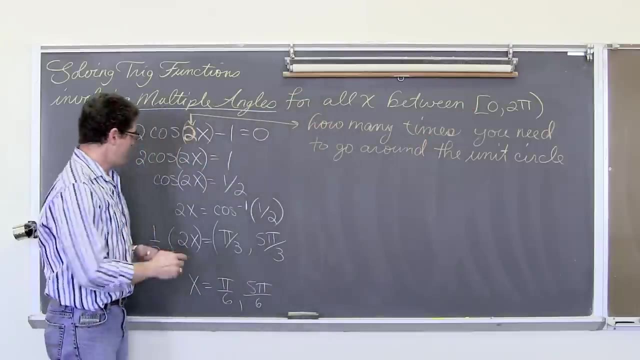 that are within 0 to 2pi. Now it says that x needs to be between 0 and 2pi, not your final answers. So we are not looking to do the inverse cosine of 1: half around the unit circle. just once all the answers that are around that first rotation of the unit circle. 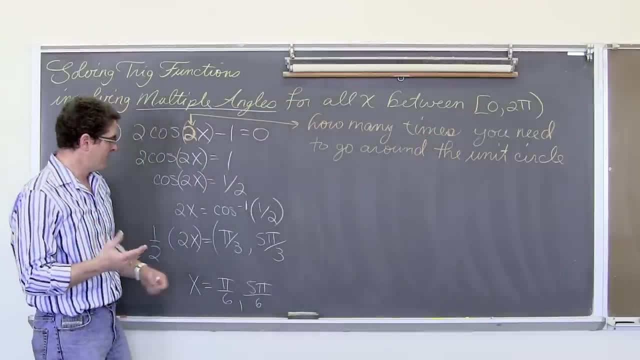 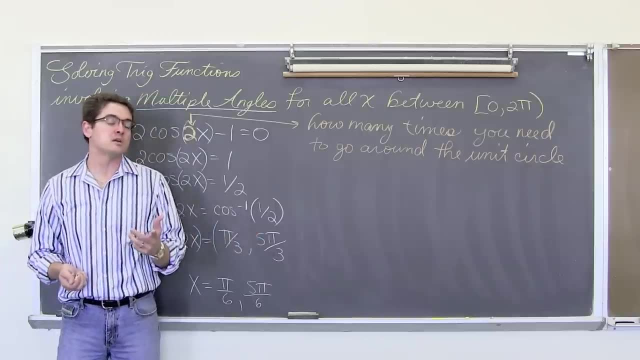 but we are going to have to go around twice to get all of the possible answers. So now you are bringing in an old concept of coterminal angles. We have already got the two places around the unit circle where cosine is equal to 1: half, but where are the other two? Well, 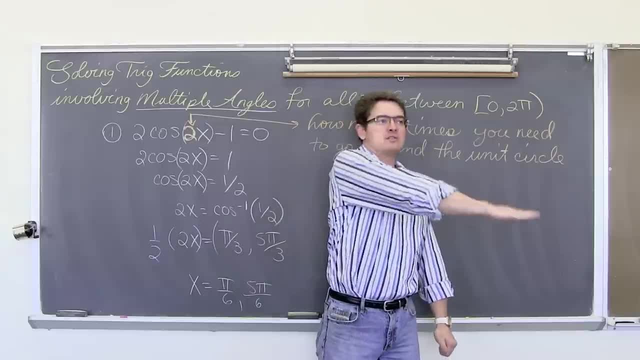 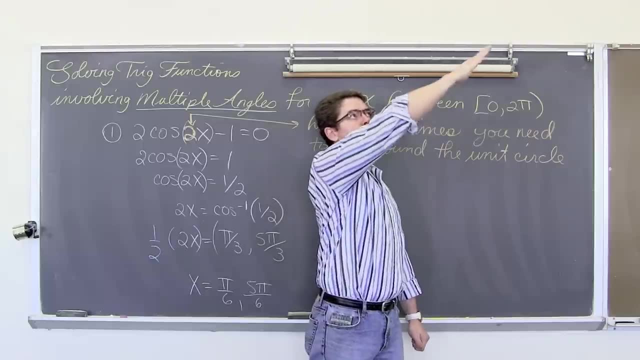 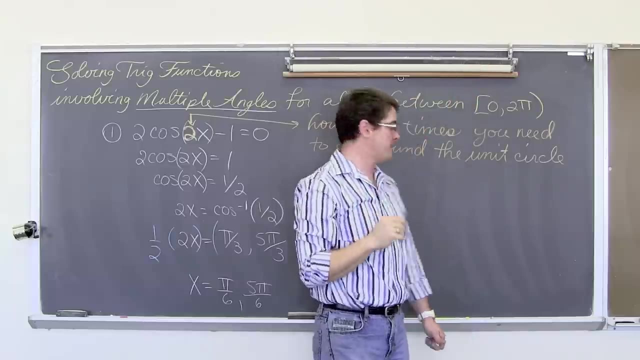 one way to figure this out is to simply count out again. Like, our first answer was at pi over 3, so I can just make another full rotation and land back at pi over 3.. So I am going to get 1,, 2, 3pi over 3,, 4,, 5,, 6, 7pi over 3.. So the other answer is going to be 7pi over. 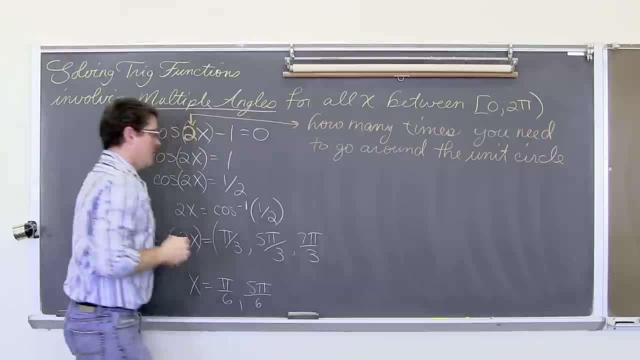 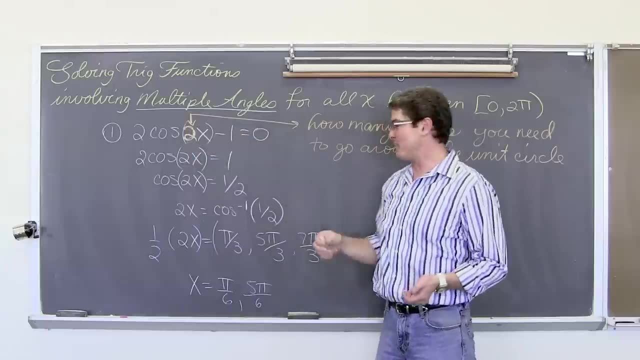 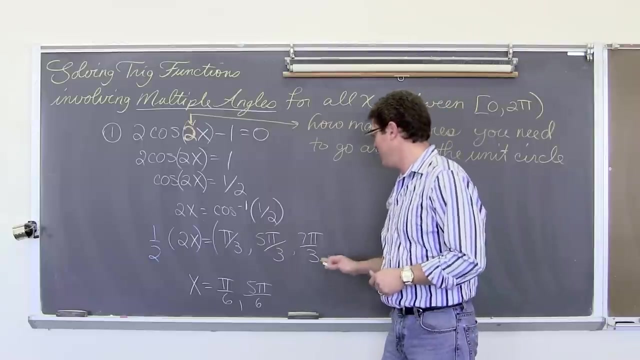 3. Now, if you have a really large multiple and maybe you don't want to just swing your arm around or put a bunch of tick marks on your paper, the only other option to find a coterminal angle, of course, is by adding by 2pi. So if I want my fourth possible answer, 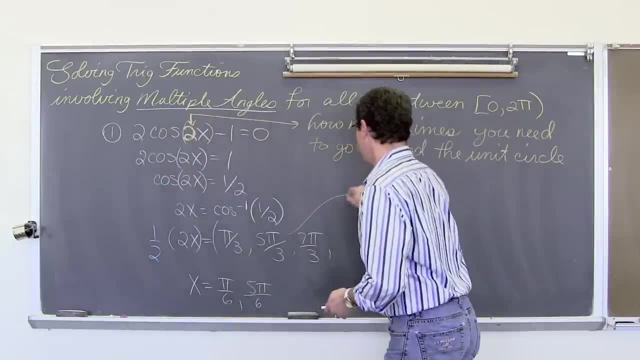 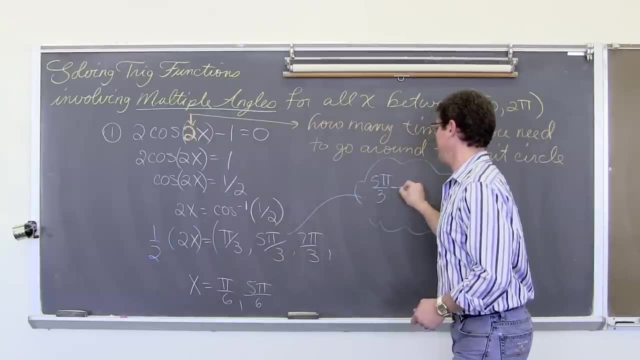 and to show you another possible answer, I am going to add 2pi over 3.. So I am going to do another way of doing this. You have to come off to the side of your scratch paper and do what is 5pi over 3, and let's add another full rotation of 2pi. Well, you are going to 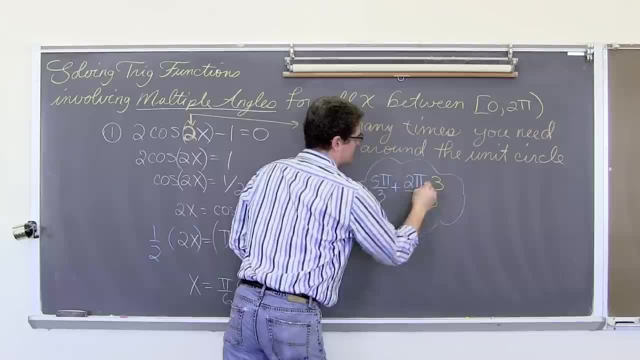 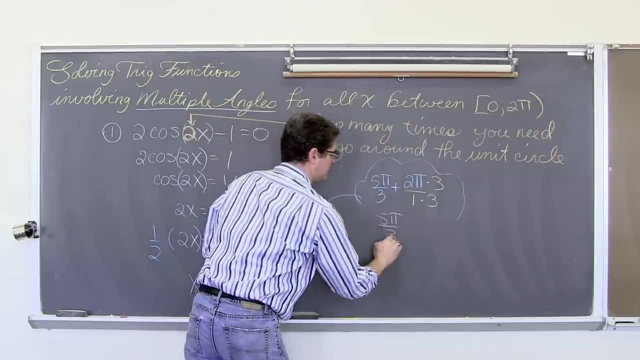 need a common denominator. So I am going to multiply the top and bottom by 3, and we get 5pi over 3 plus 6pi over 3.. Ok, so my other possible answer is going to be 5pi over 3.. 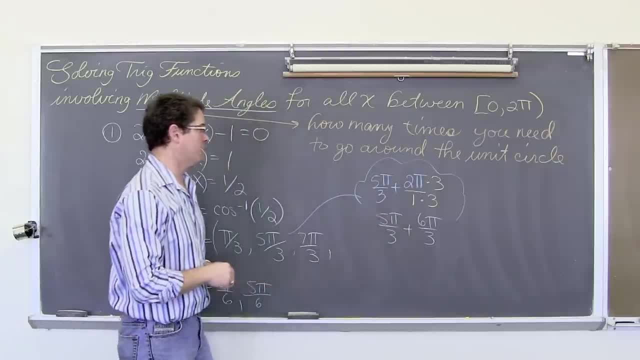 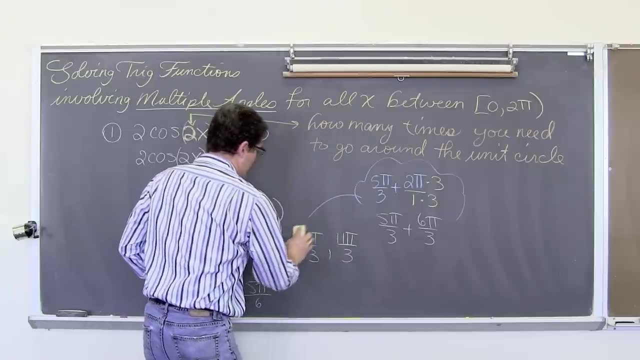 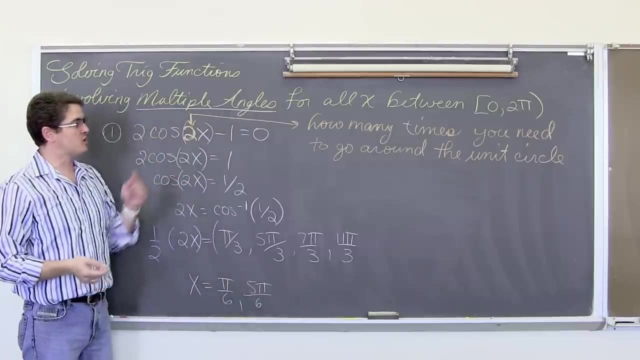 So my other possible answer, therefore, now that we have a common denominator, is 11pi over 3.. So we have again the idea, the new idea of Saldini's equation with trig functions, when you have a multiple angle is just to remind yourself that multiple on the angle 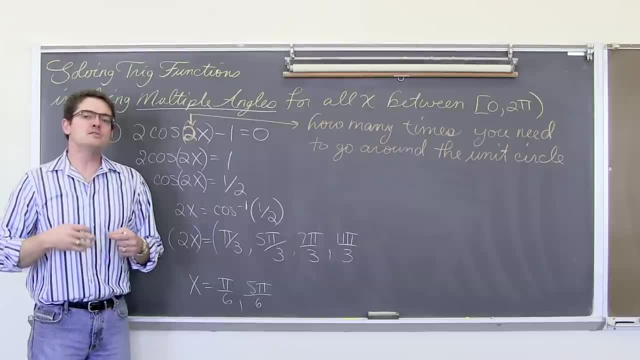 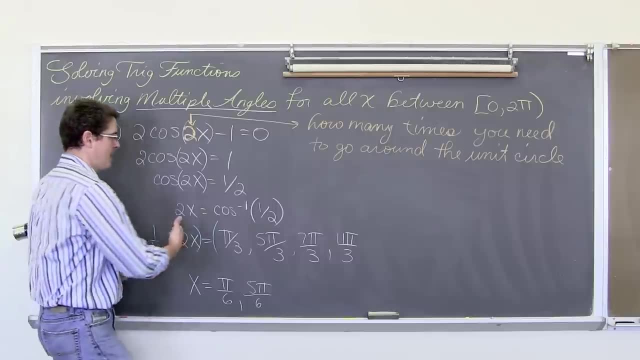 is simply telling you how many times you need to go around the unit circle so that, when you are done, you have all of the possible answers that are required based on the directions. So now we have four possible answers from going around the unit circle twice and you 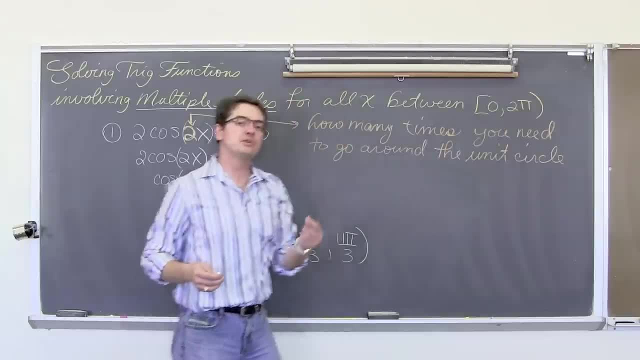 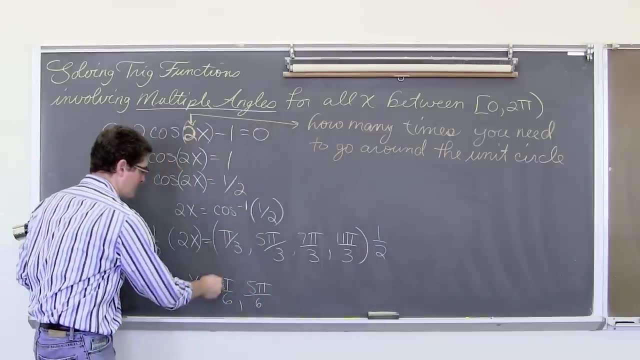 know 7pi over 3 and 11pi over 3 are bigger than 2pi. but I have to finish my last step, which is multiplying both sides of this equation by 1 half. Now we have the pi over 6, we have 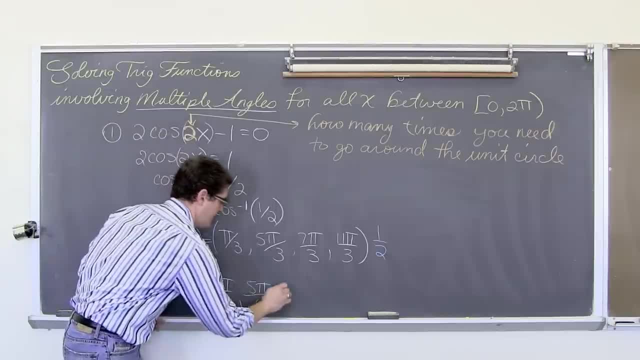 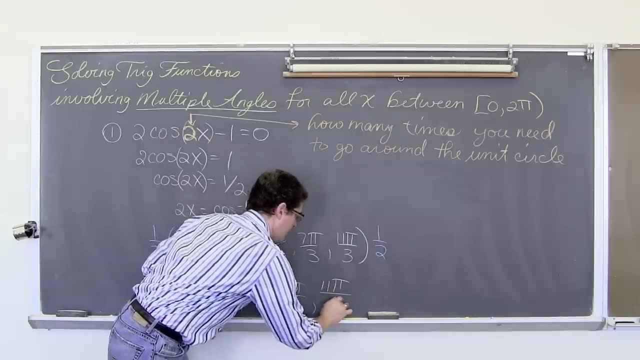 1 half times 5pi over 3, which is 5pi over 6, and then 7pi over 6 and 11pi over 6.. This is not always going to happen. All of these answers here are on the unit circle and we are comfortable knowing that. 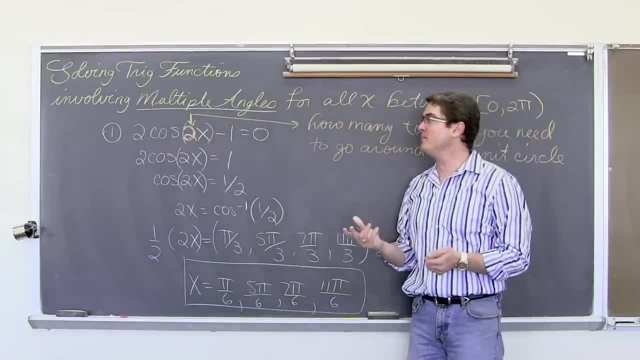 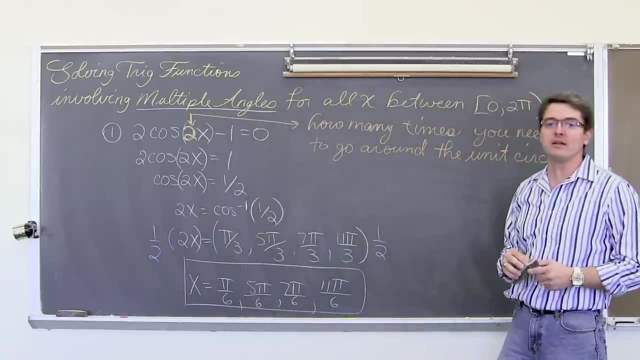 all of those are definitely, indeed, less than 2pi. So again one last time before we deal with the last three examples with multiple angles. that tells you how many times to go around the unit circle to find all of your answers. So a couple more examples. 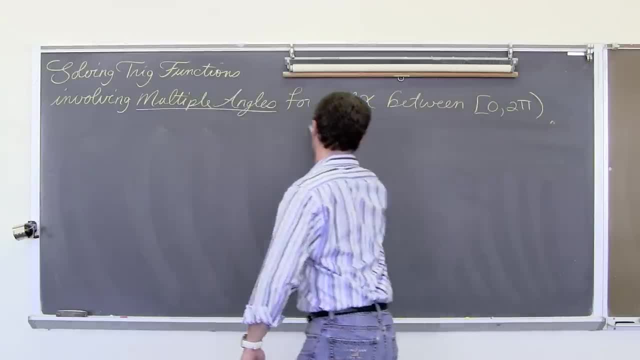 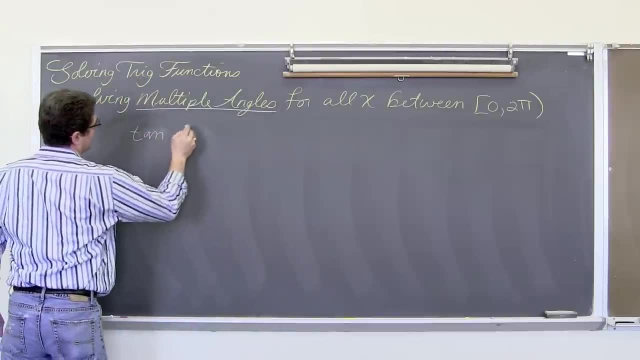 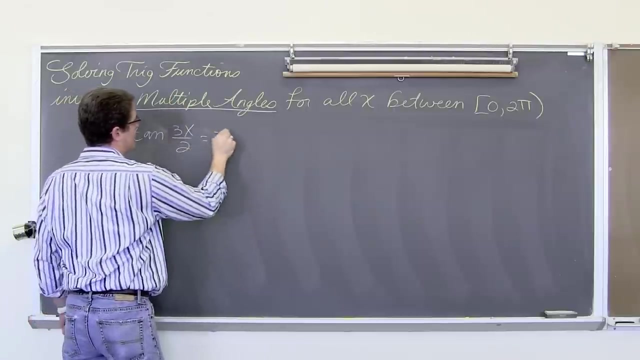 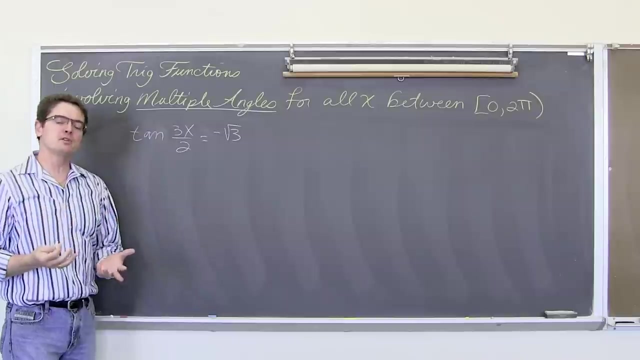 Orange chalk is not wanting to erase very good. Okay, so we have tangent of 3x over 2 is equal to negative square root of 3.. Well, this one is already set up. The only oddity is this whole 3 over 2.. Well, 3 over 2 is 1.5, so we are going to want to go around the unit. 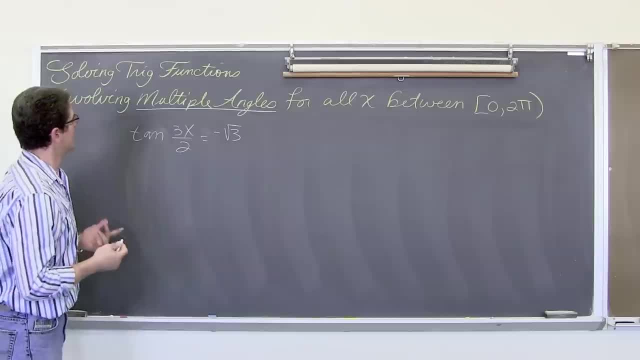 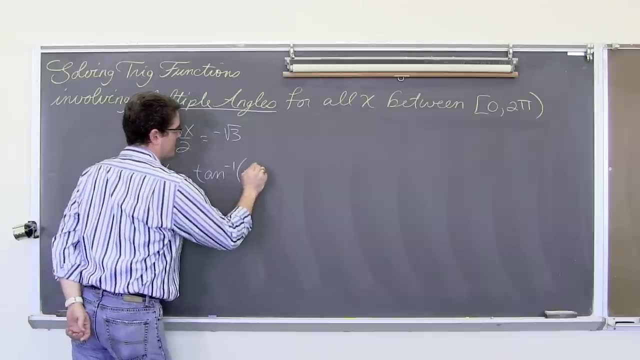 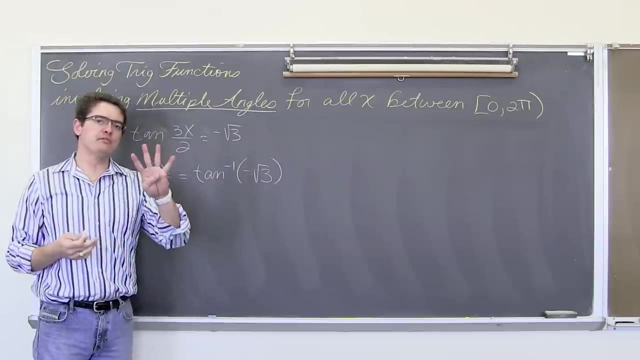 circle 1 and a half times to get all of our possible answers, possible answers that we want. So 3x over 2 is equal to the inverse tangent of negative square root of 3. Tangent is negative in quadrants 2 and 4.. So what first answer do we have? 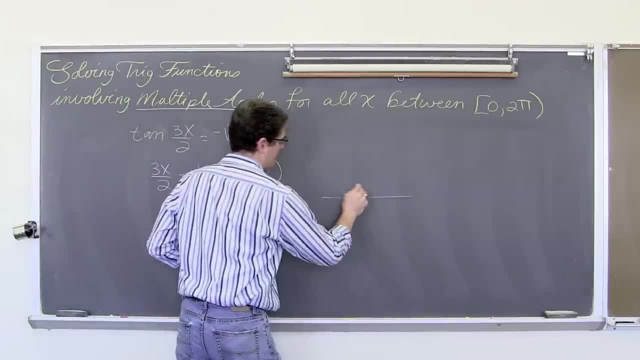 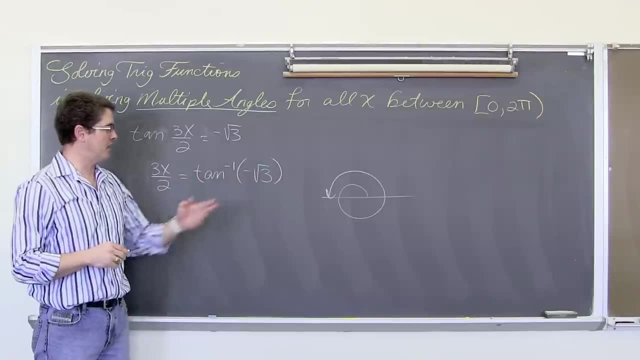 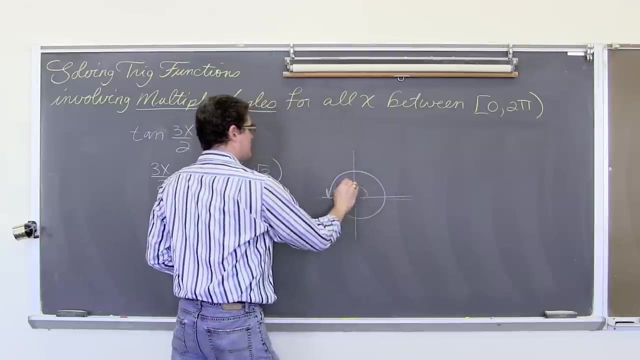 What first angle do we have in our first one and a half rotations? that puts us in quadrant 2? Where, of course, tangent is negative square root of 3.. Well, if you remember your unit circle, and certainly by now you have at 2pi over 3, your coordinate is negative one. 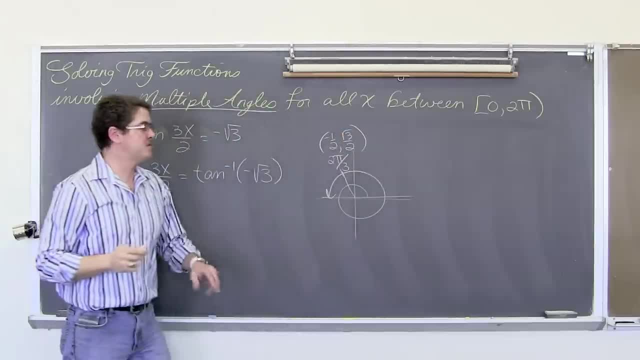 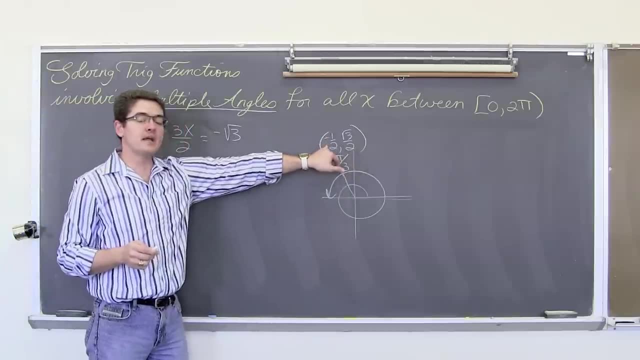 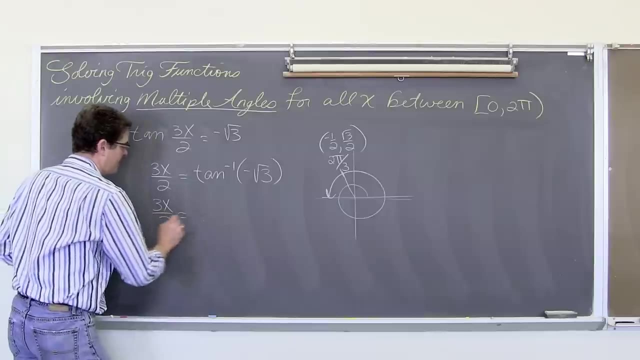 half square root of 3 over 2.. When you take that y over x, the ratio for tangent, the y value of square root of 3 over 2 over negative one half does cancel out to be negative square root of 3.. So our answers here are going to be 3x over 2.. First answer is 2pi over 3.. 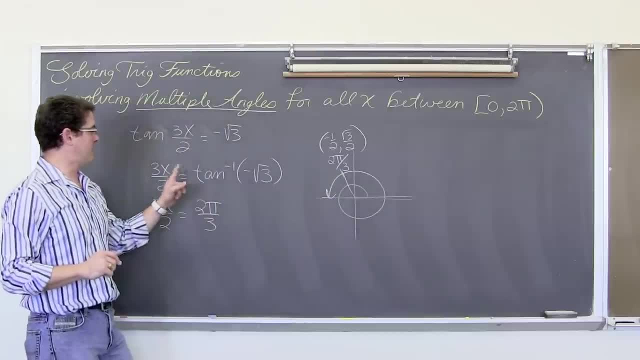 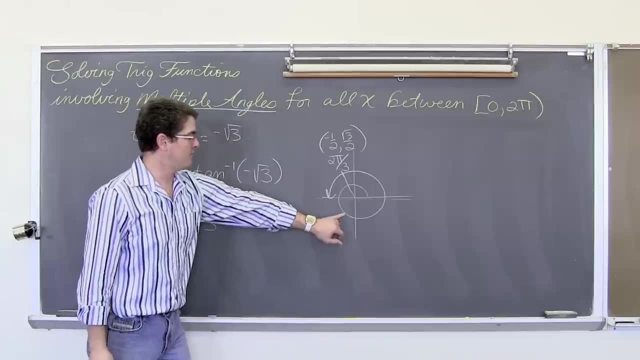 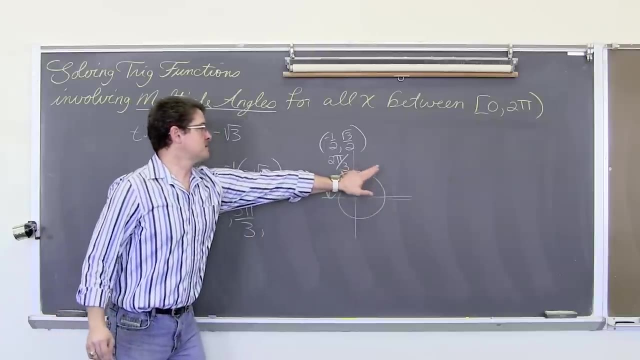 And then, with that first one and a half rotations, we are again getting from the multiple of three halves, 3 divided by 2.. We have 2pi over 3, 3, 4, 5pi over 3,, 6,, 7, 8pi over 3.. 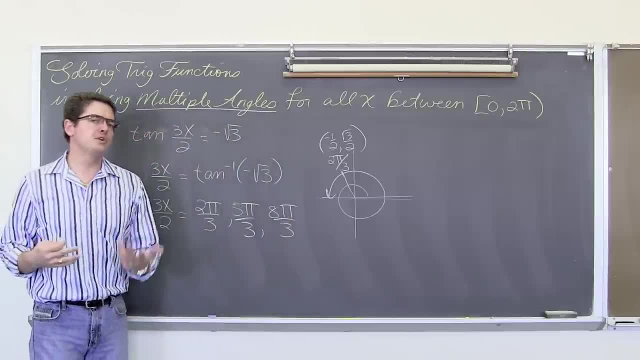 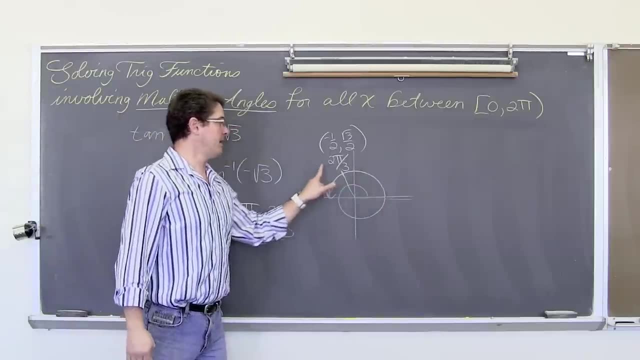 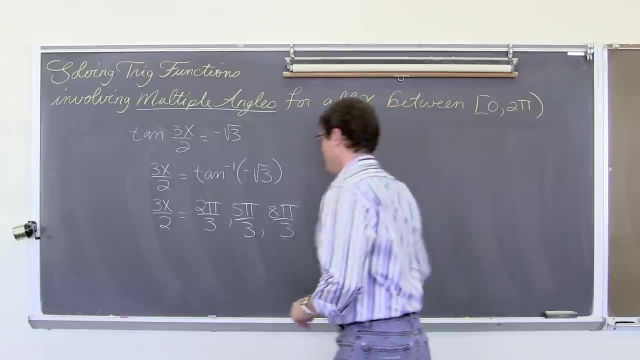 And I don't need to go around two full rotations again, because my multiple is three halves or 1.5.. So we need to go around the circle, the unit circle, one and a half times. And these are my three possible answers. So our last step is to get that x value alone, which? 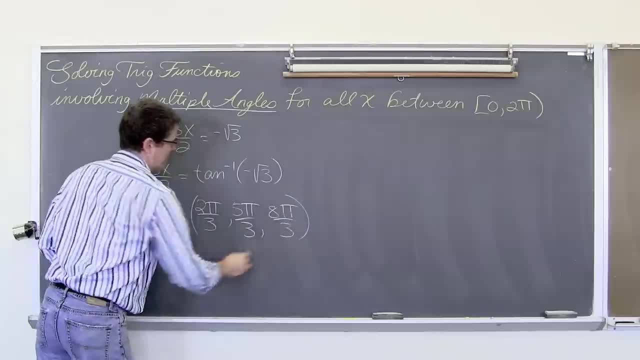 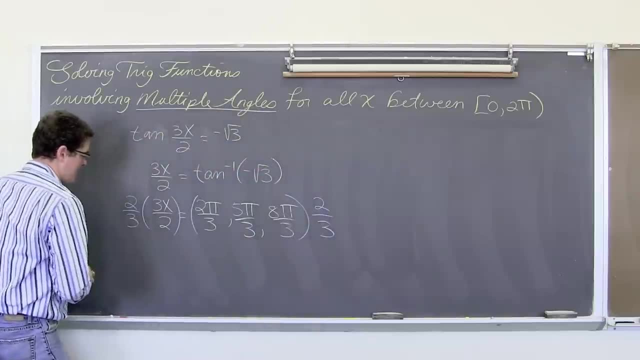 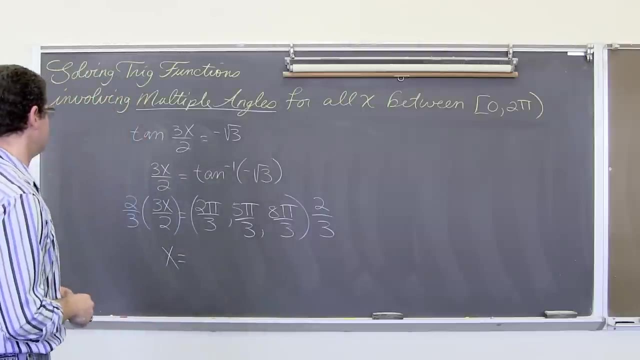 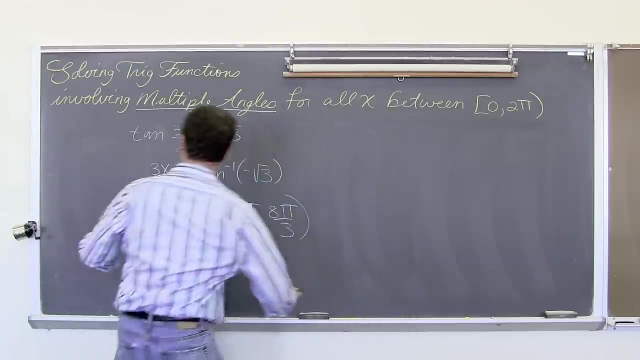 means we are going to need to multiply both sides of this. Well, it is not really an equation, it is just a list of answers. But multiply everything by 2 thirds, That cancels out. So x is equal to Well, 2 thirds times 2 thirds is Yes, 2 thirds Is equal to. 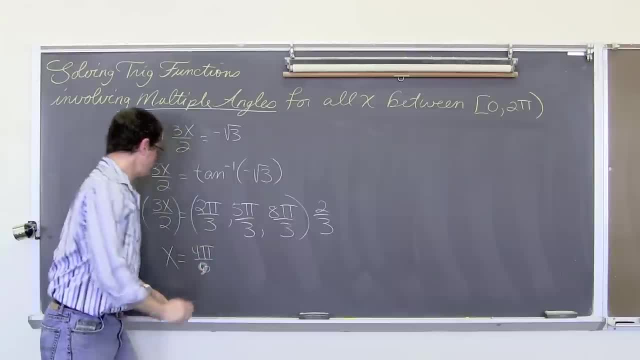 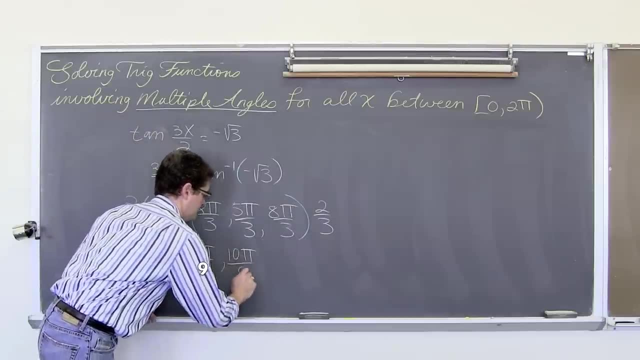 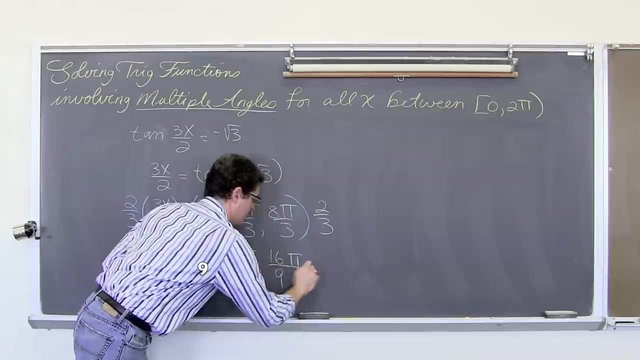 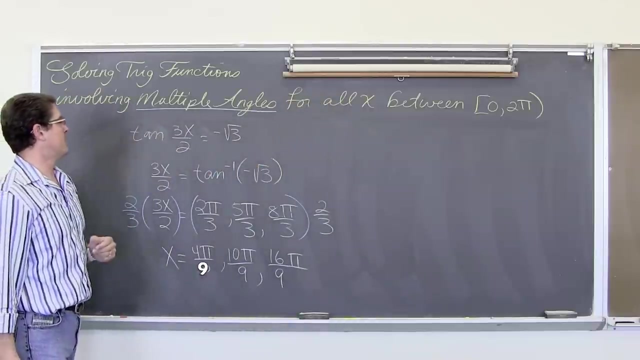 4 over 6.. And 2 times 5 is 10 over 9.. And 2 times 8 is 16.. Oh, 9.. 16pi over 9.. So there we go, Our three answers: between 0 and 2pi. for the tangent of 3pi over 2x equals negative square root. 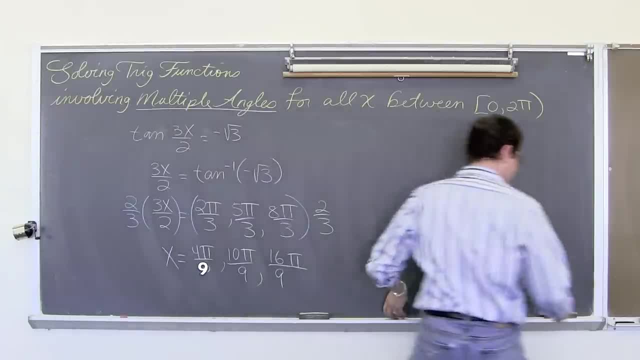 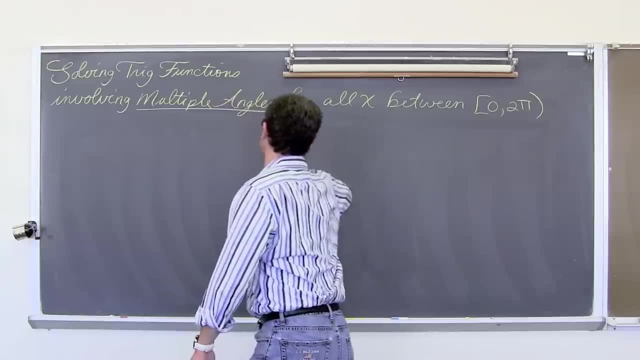 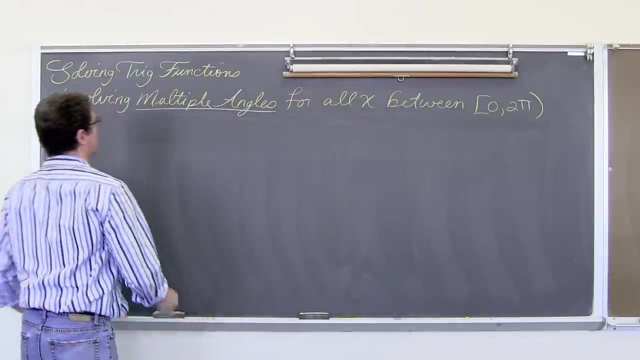 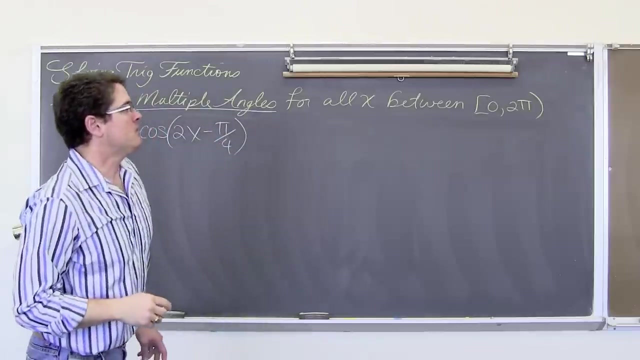 of 3.. Ok, let's go on. Ok, For our next example, let's take a look at: No, No, No, No, No. look at: the cosine of 2x-pi over 4 equals square root of 2 over 2.. Alright, so this. 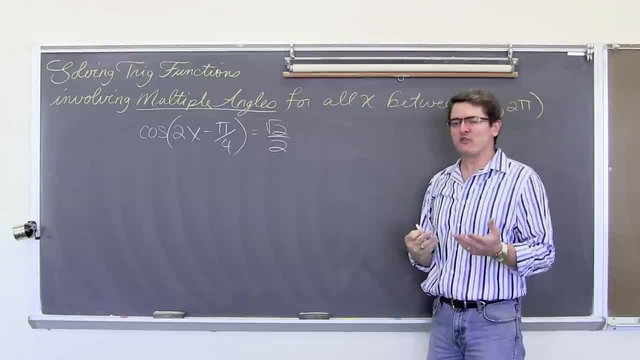 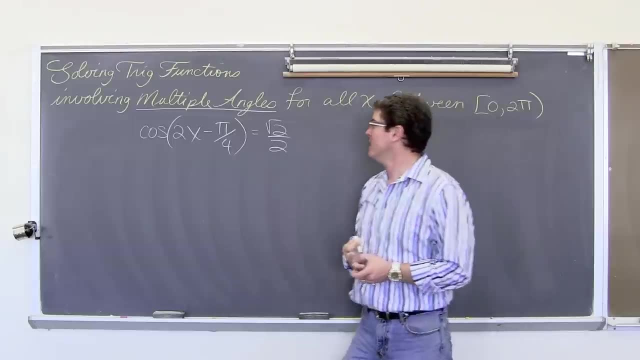 is kind of a funny looking angle: 2x-pi over 4.. I think we are going to have to go around that unit circle two times and let's just see how the negative pi over 4 works out. Well, we are going to have to get our cosine function away from the angle measure, as always. 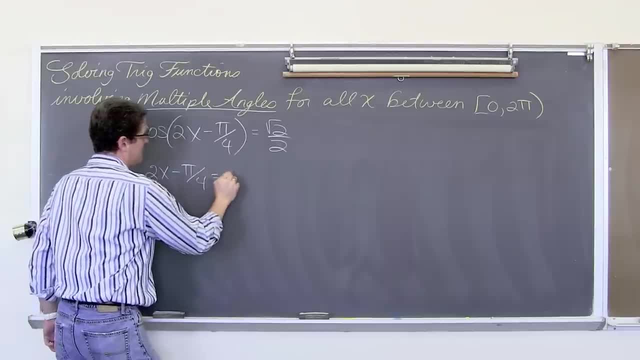 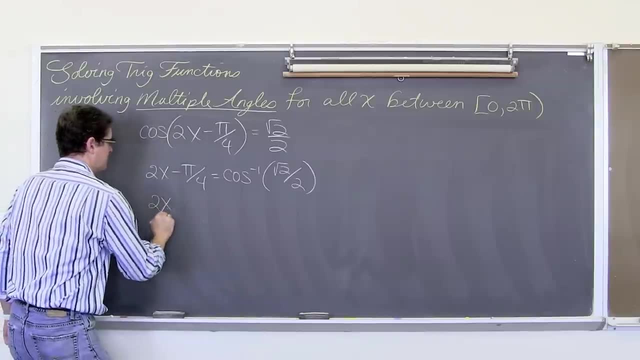 So 2x-pi over 4 equals inverse cosine of square root of 2 over 2.. That means we are going to have 2x-pi over 4 and inverse cosine of square root of 2 over 2, where on the unit 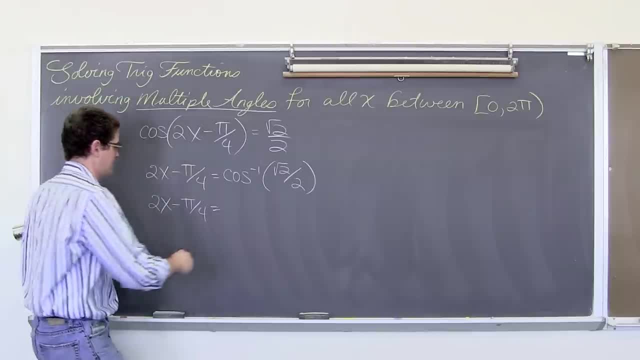 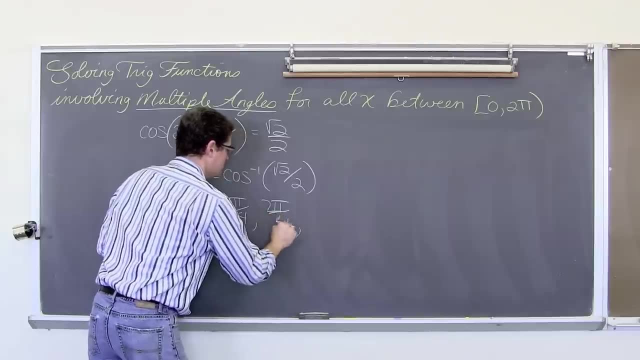 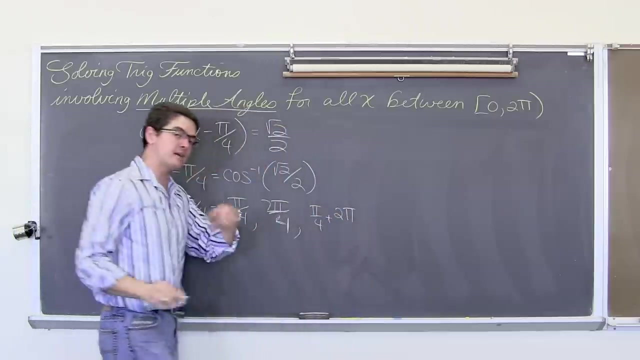 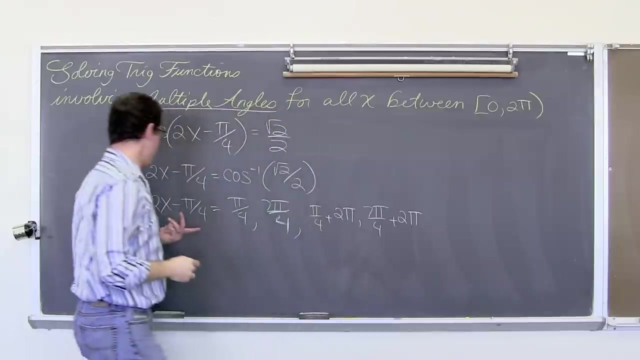 circle. is cosine equal to this ratio, That would be at pi over 4,, 7pi over 4,. and then how about pi over 4 plus 2pi to get that next rotation in, and 7pi over 4 plus 2pi, So that 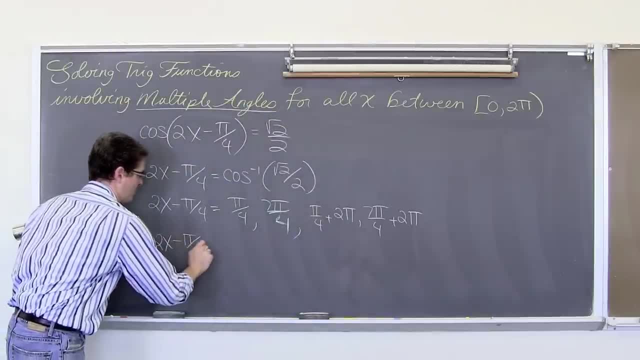 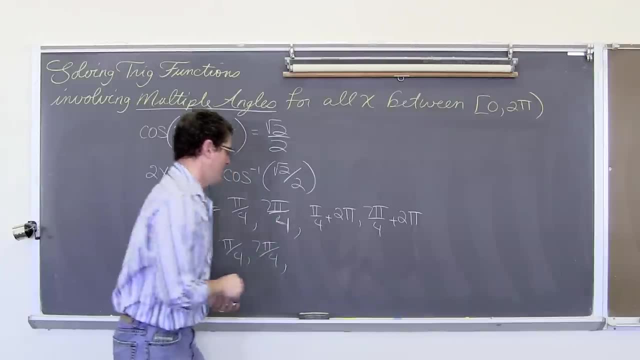 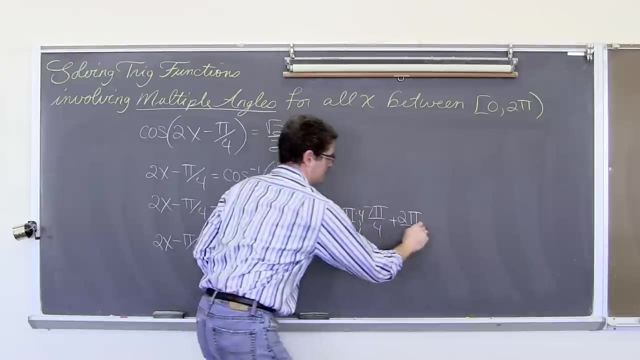 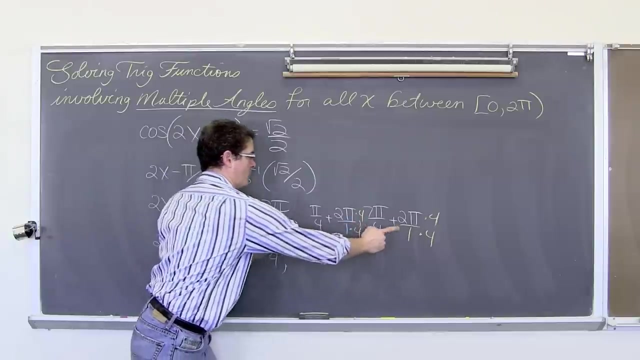 is going to give us 2x-pi over 4, equals pi over 4, 7pi over 4.. Find a common denominator here. just showing you some other ways to work these out And again just reemphasizing that when you go one full rotation away, that is the idea. 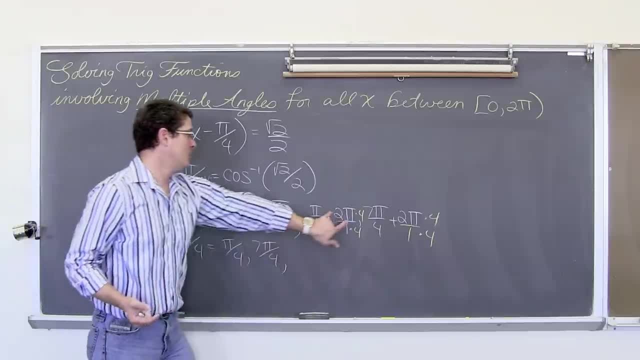 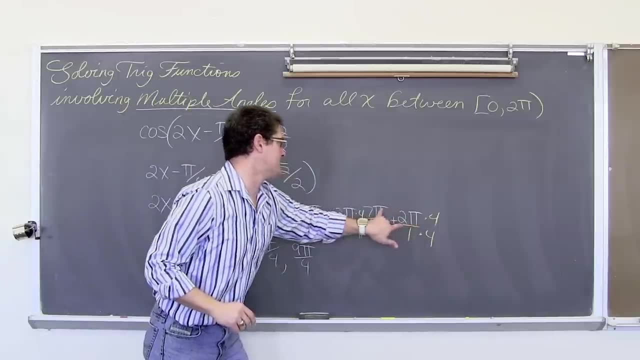 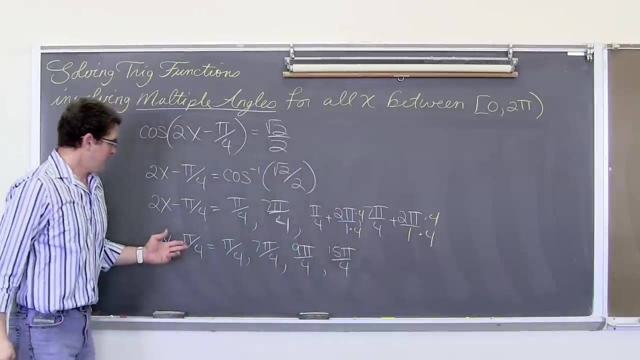 of coterminal angles. Those are when the trig functions are equal. So we have 8 plus 1 is 9.. And finally we have 2 and 4 is 8, and 7 is 15.. Now let's deal with this. pi over 4. 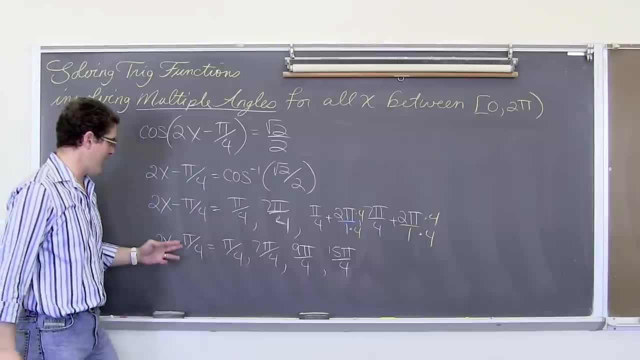 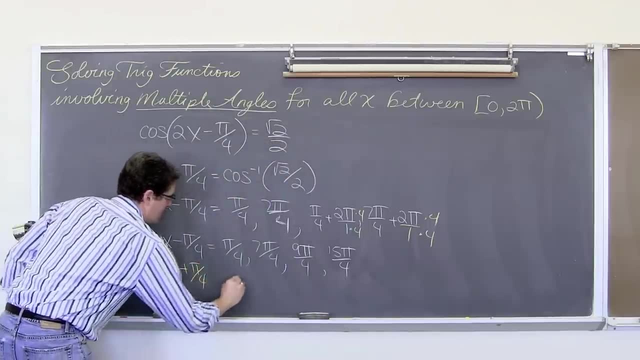 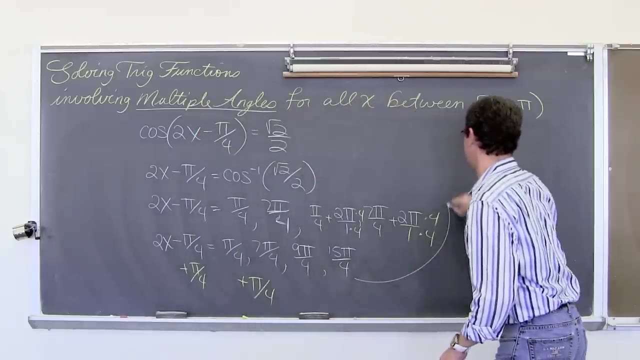 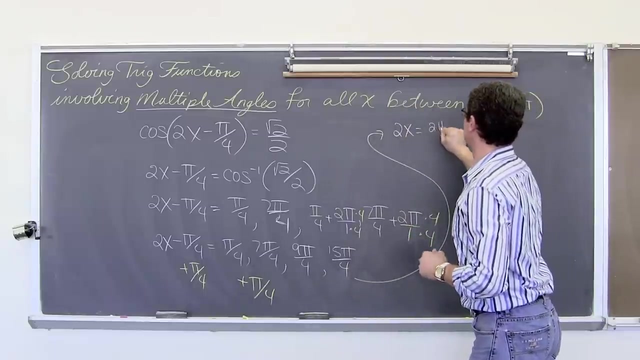 is over here. Well, I have got to move it over and add pi over 4 to all of these answers. So I am adding by pi over 4, and I am also running out of space, So we are going to have: 2x is equal to 1 fourth and 1 fourth is 2 fourths times 7: 4 and pi over 4 is 8pi. 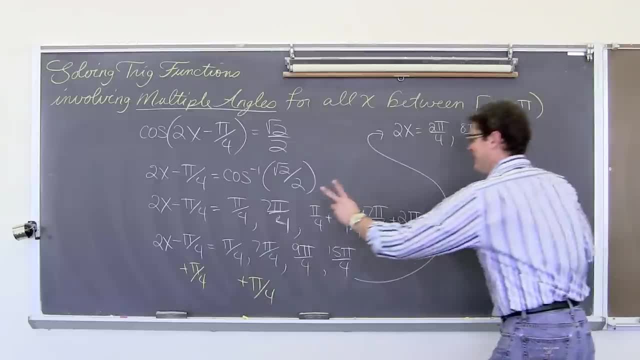 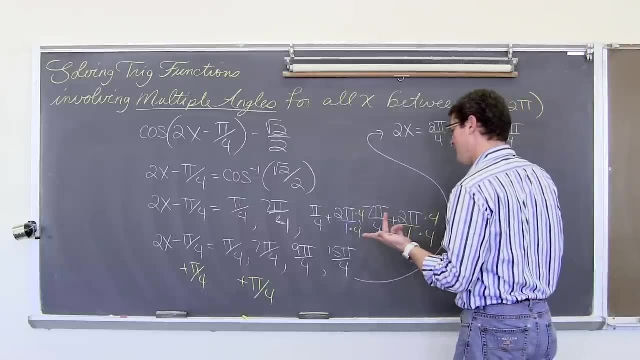 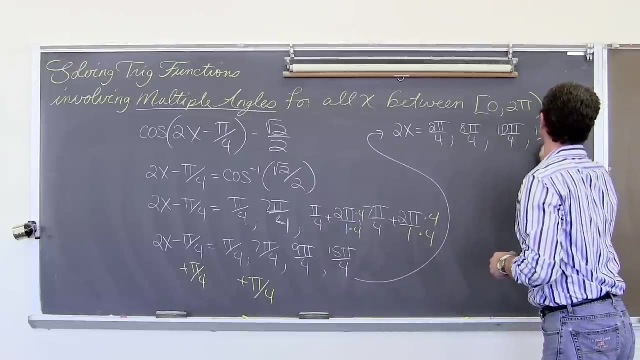 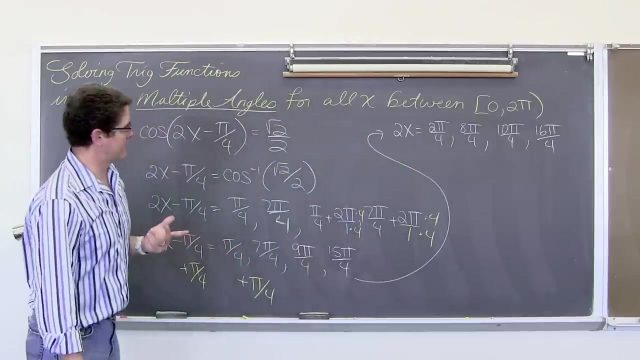 is 8pi over 4.. 9pi over 4 plus 1pi over 4 is 10pi over 4.. Pi over 4 plus 15pi over 4 is 16pi over 4.. Ok, so our last step is to divide everything by 2 or multiply both sides. 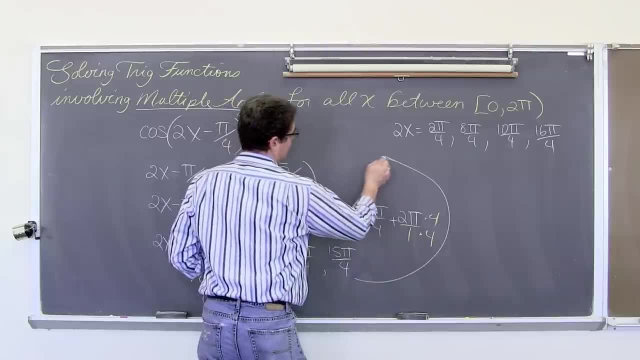 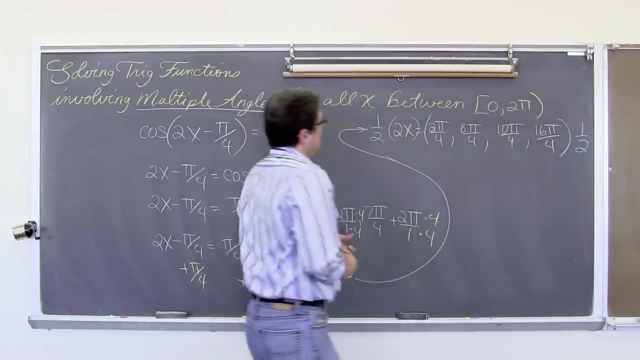 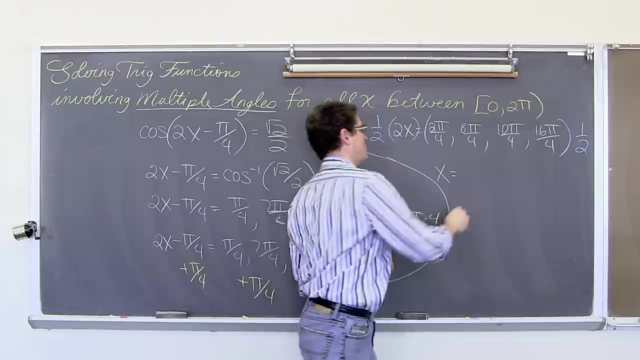 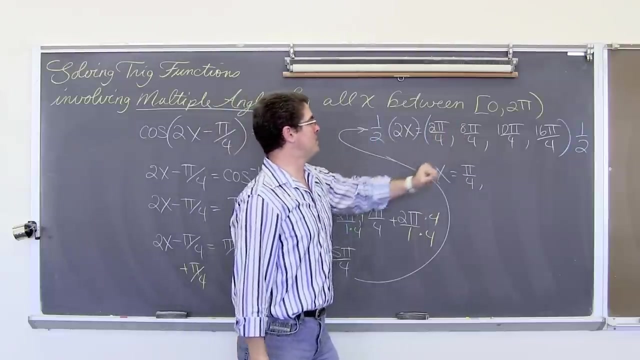 of this sort of lists of answers. This is sort of an equation. And multiply everything by 1 half, What do we have? Say x is equal to 2 divided by 2 is equal. pakina m 2 is 1, so pi over 4 is 1.. 8 divided by 2 is 4.. 4 over 4 is equal to 1.. Then we have 10 divided. 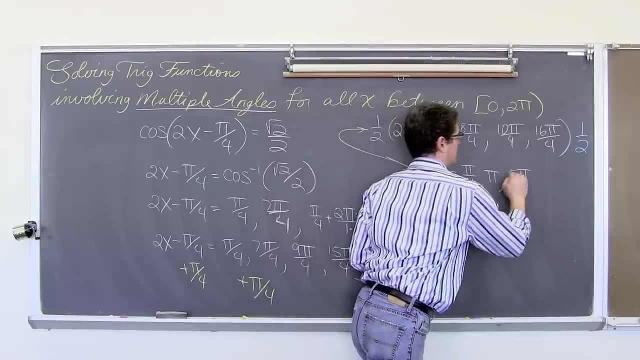 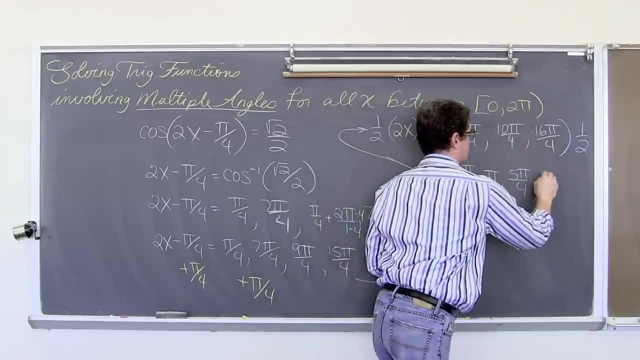 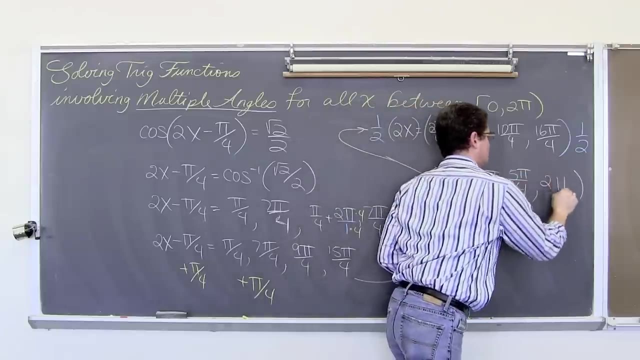 here by 1 is 37.. There we go, Finally. now I have this就解除10 really. So, whatever, 2 is 5,, so 5pi over 4.. 16 divided by 2 is 8, and 8 divided by 4 is 2pi. Now remember. 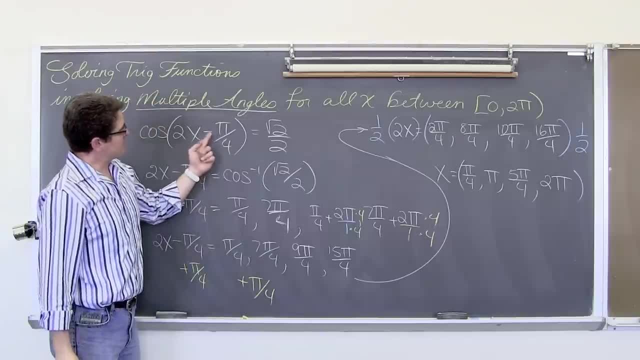 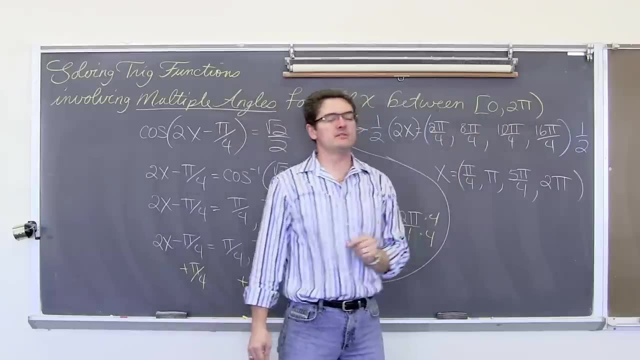 that negative pi over 4 thing there, Because that minus pi over 4 is there. if you look and make sure that you want to make sure that all of your final answers are actually within the restriction given to you by the directions. Of course I have 2pi. it is in the interval. 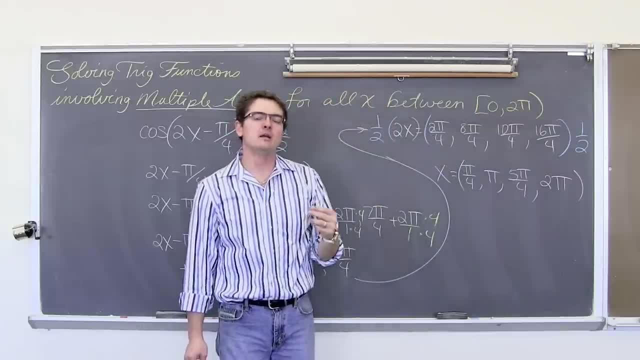 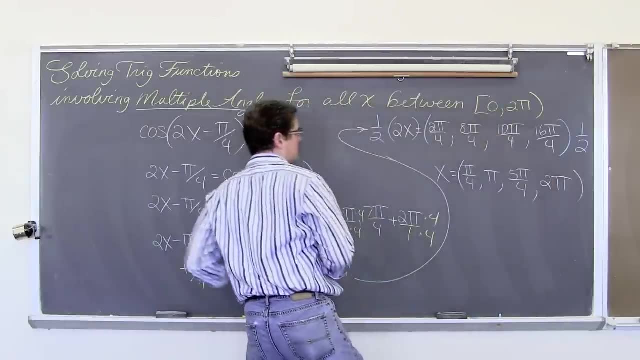 but I have a round parenthesis here, which means I want to go up 2pi but not actually included. So that subtraction there is causing us to make sure to say: hey, don't forget to double check your answers. I basically just went a little bit too far and got one extra. 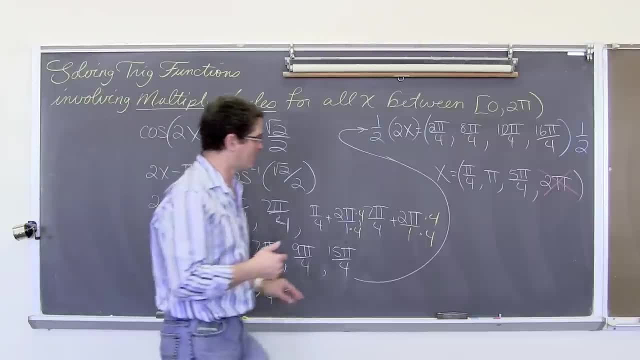 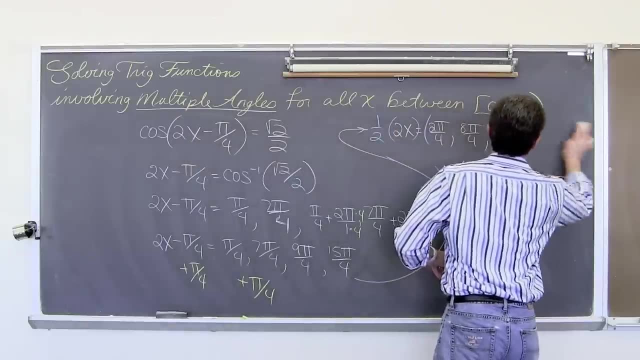 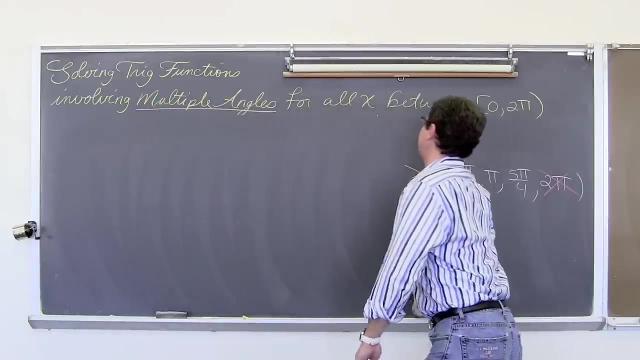 answer that I didn't need or want. Alright, so one last example, and we are going to call this video a day. Let me double check to make sure I have that right. Yep, So I am going to double check my answers. One last example, and this example is going to give me lots. 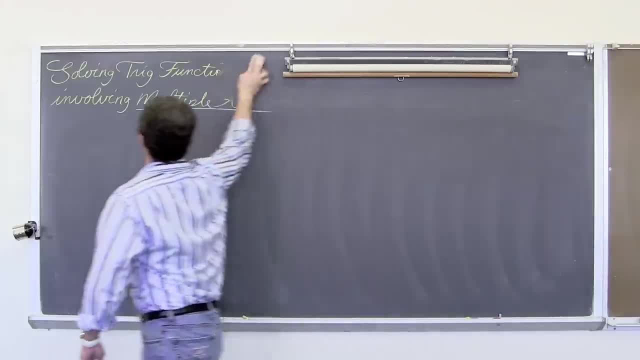 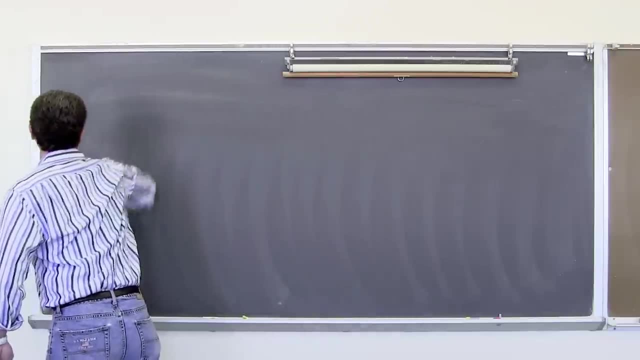 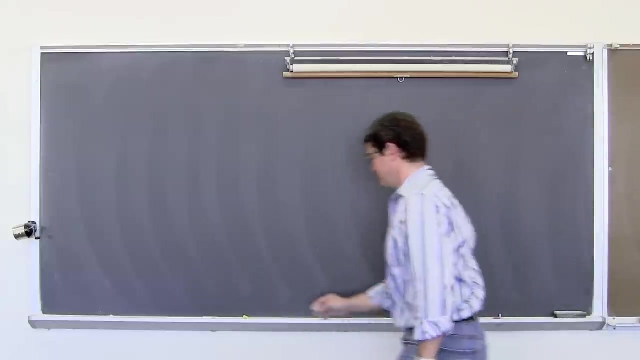 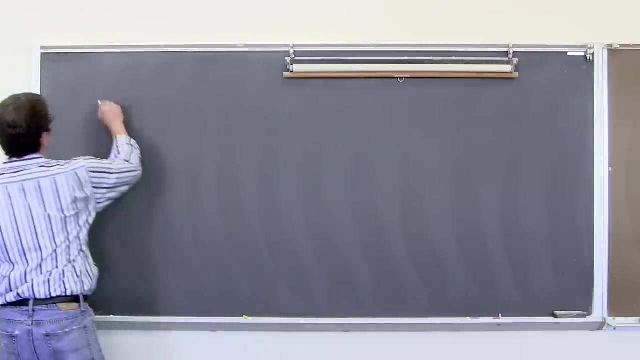 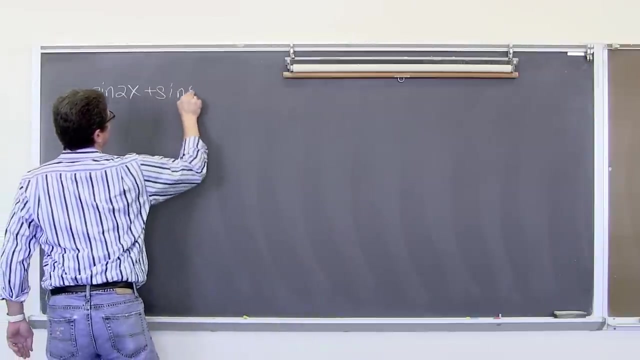 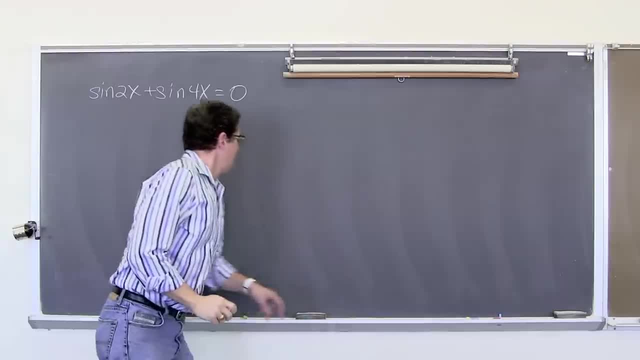 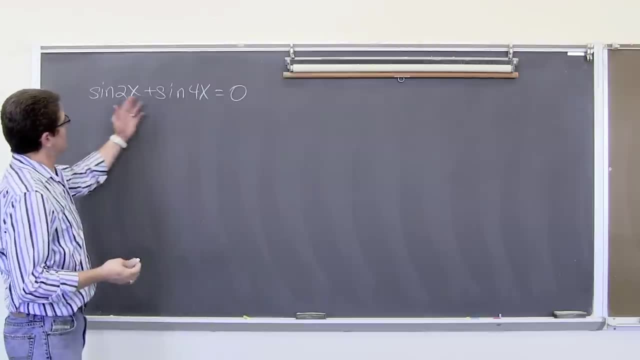 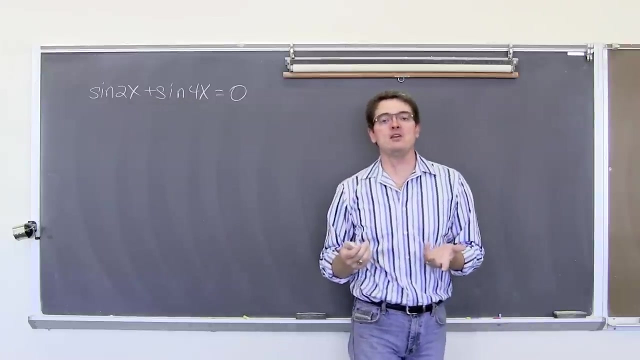 zero. Ok, Well, we have to solve this. How are we going to do that? Because we also have multiple angles here, but they don't even match. Now that is a problem. This is effectively like having two variables in the same equation, So unless we can factor those apart and do, 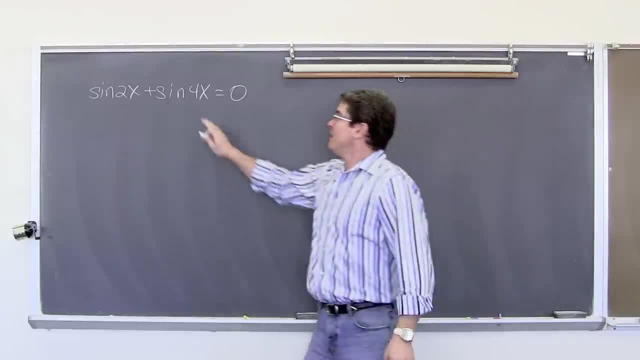 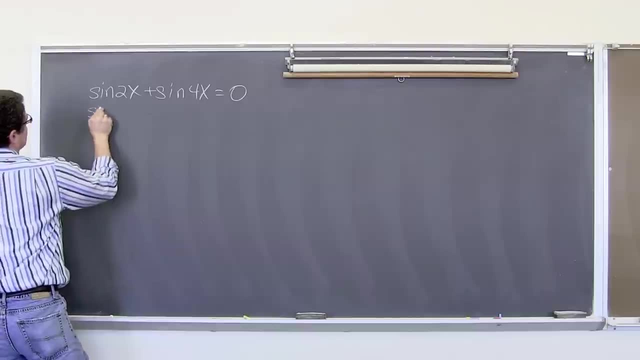 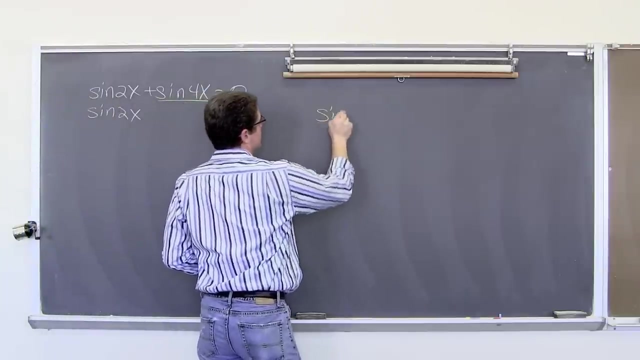 something with our identities. this is not going to be solvable, But if I use a double angle identity for sine to reduce this down, I will have something that I can actually solve. So we have the sine of 2x and the sine of 4x. I am going to use this identity. 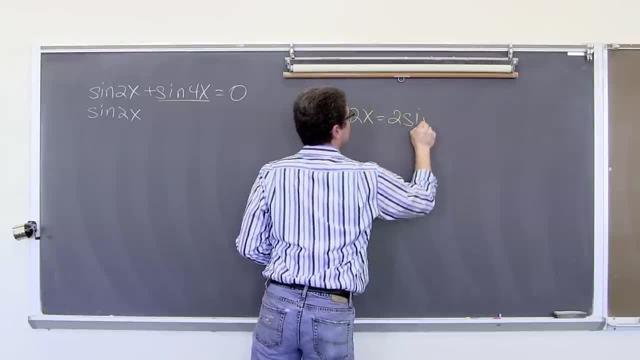 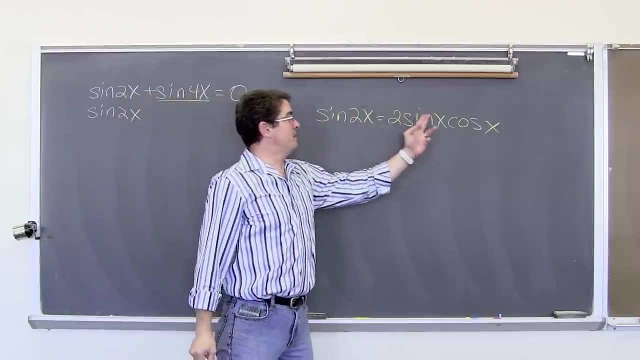 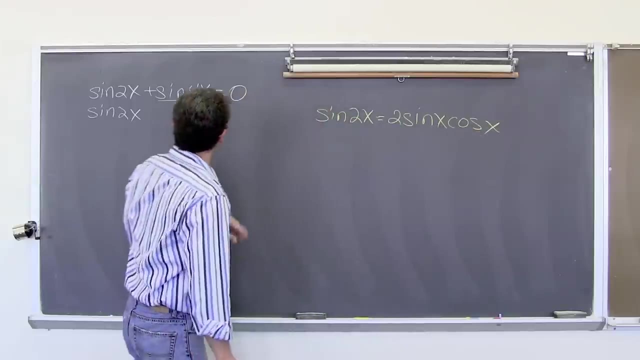 The sine of 2x is equal to 2 sine x, cosine x. Ok, It is not so important that this is 2 and this is 1x. What is important is, this angle is double what these two angles are. So I have a 4 here instead of a 2.. That just means. 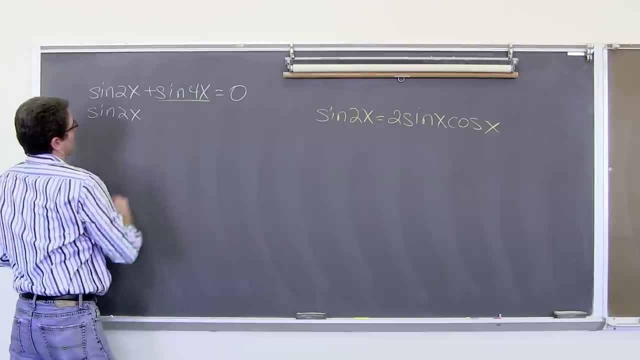 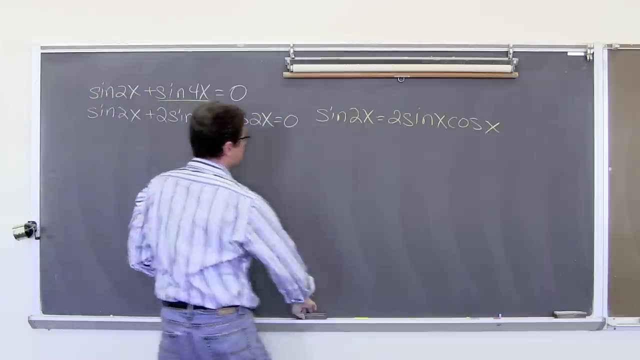 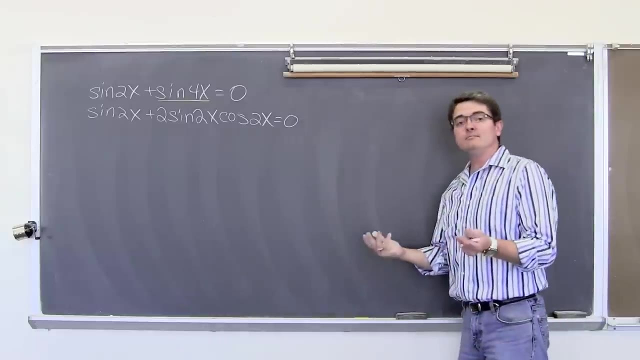 I am going to have two x's here. So the sine of 4x is equal to 2, sine of 2x, cosine of 2x equals zero. Now we still have these two equations or these two variables, but they will factor. 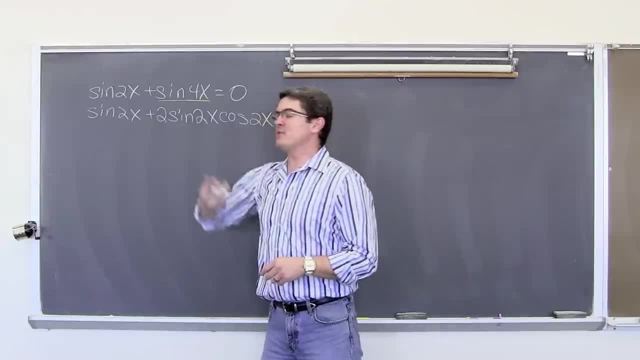 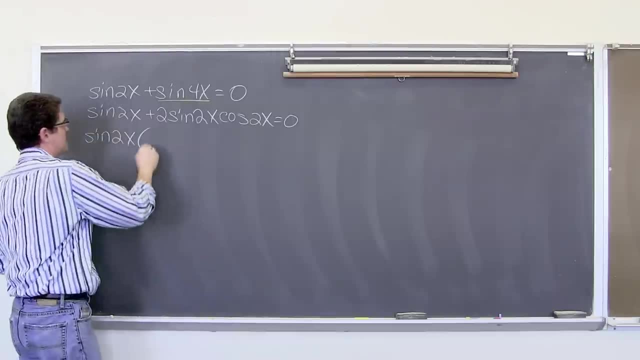 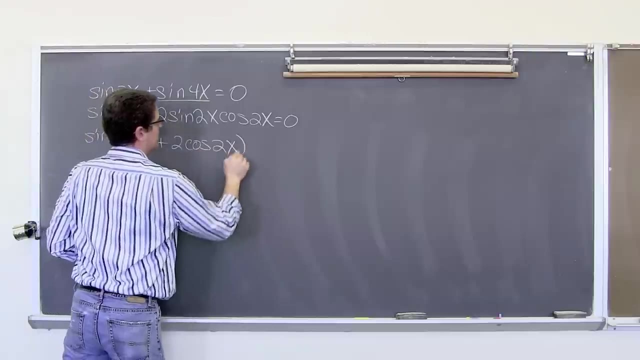 apart, and that means we can actually work this out. These two terms both have a sine of 2x. That is going to come out: Sine of 2x divided by sine of 2x is 1 plus sine of 2x divided by sine of 2x. This cancels out. We get 2. cosine of 2x equals zero. I am going. 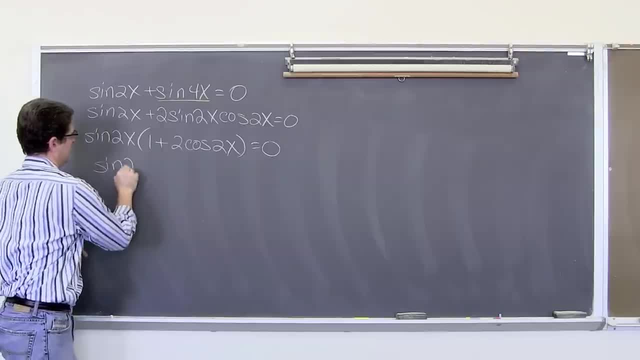 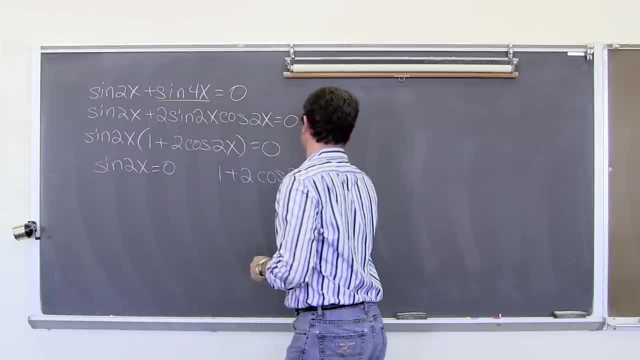 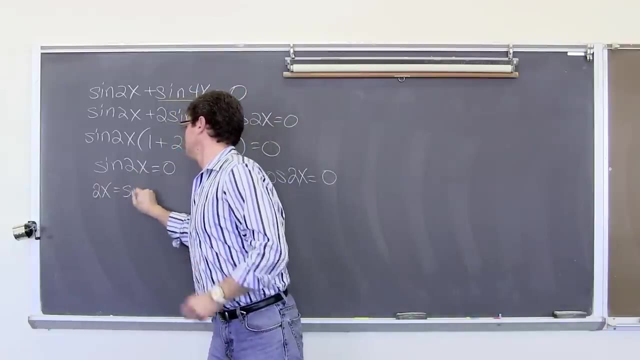 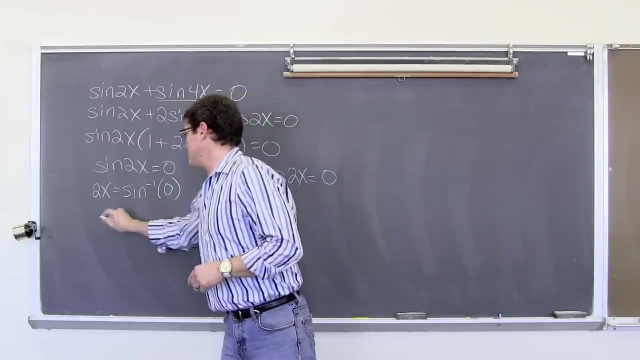 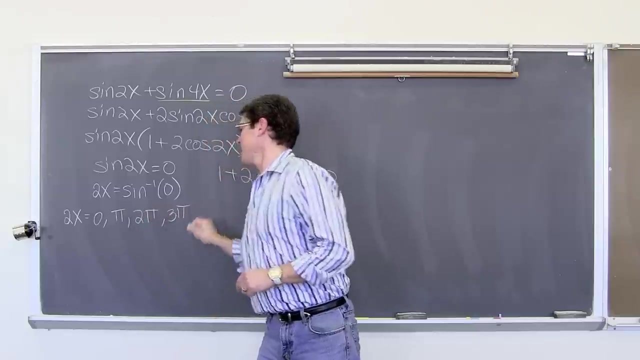 to set each one of these factors equal to zero. Solve each one. Where is sine equal to zero? Again, we are talking about a double angle, so I have to go around in a circle twice. That is going to be at 0, pi, 2pi and 3pi. 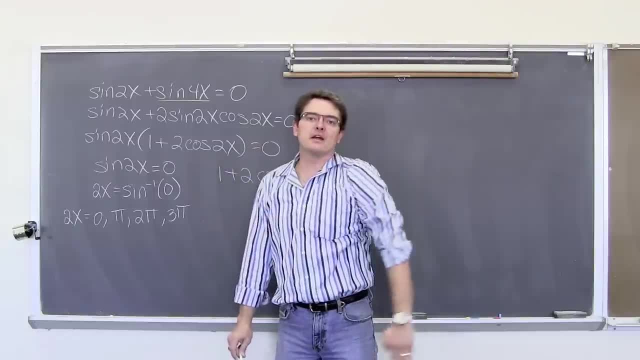 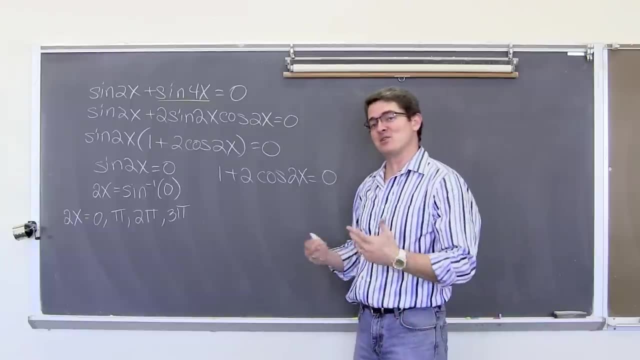 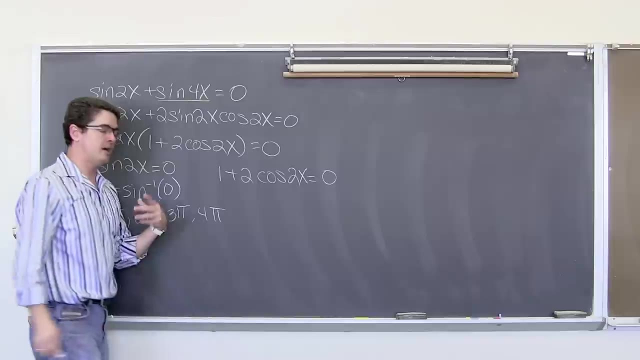 If I continue to go around I am going to get to 4pi, but that is going to be too big. because of the restriction that I raised, It has to be between 0 and up 2 to 2pi. If you add an extra one in there, you are going to notice that it is too large when you go. 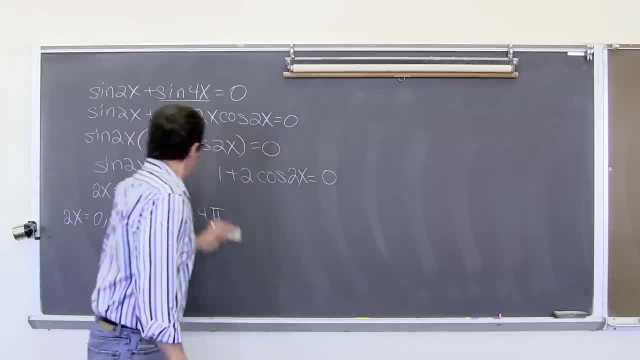 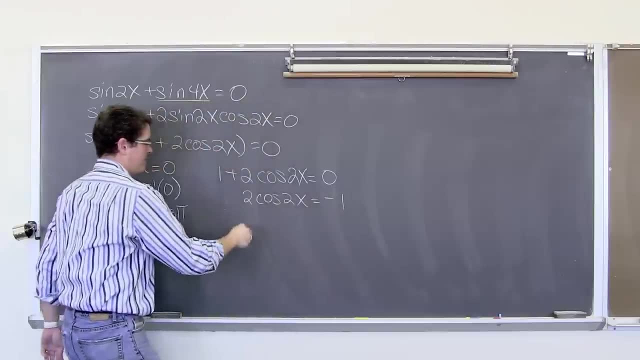 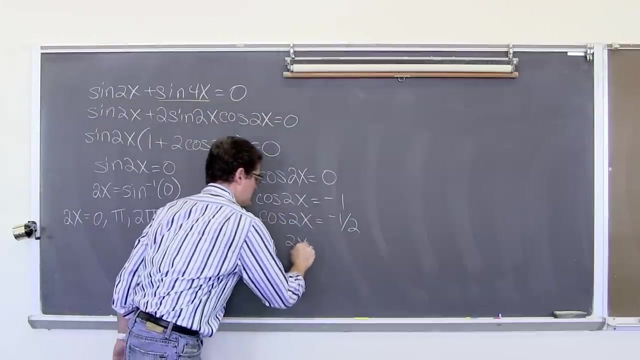 back at the end and check your answers. So we are going to subtract both sides by 1.. Divide everything by 2.. Again inverse trig function. So 2x is equal to the inverse cosine of negative 1 half.